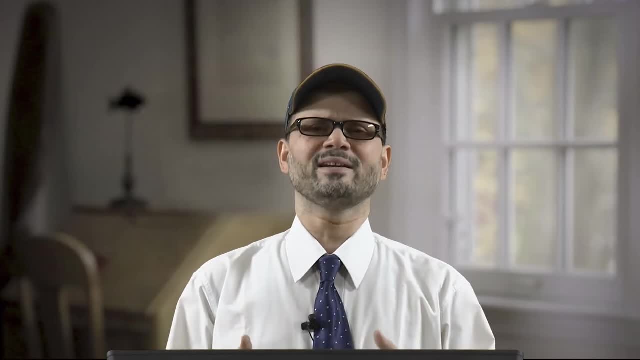 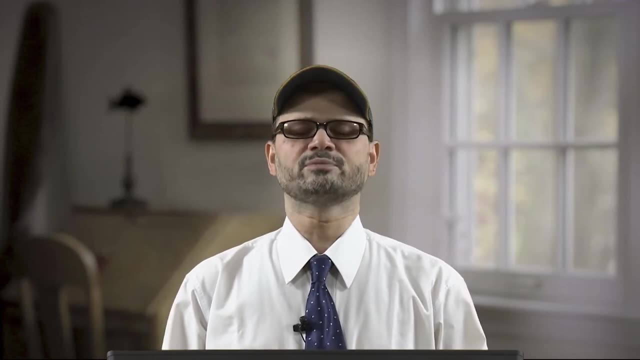 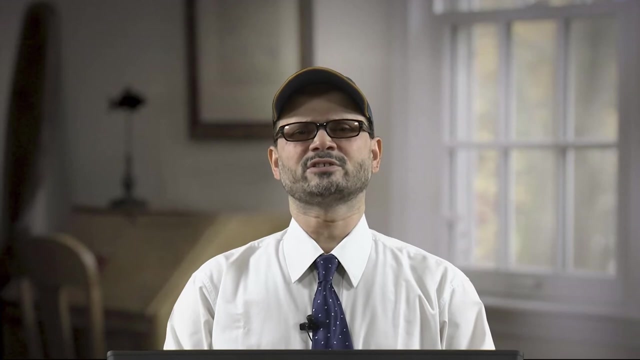 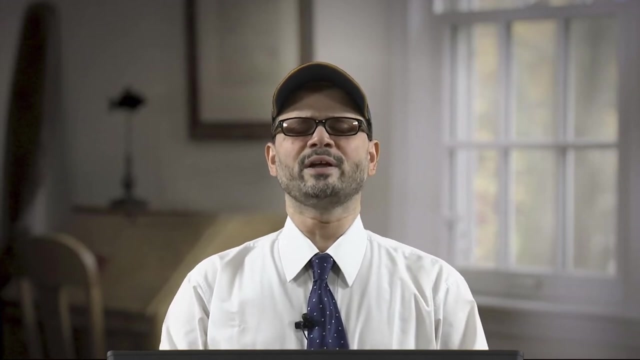 getting the near And net shape or the final shape of the product and you have a better yield. you do not have wastage, So you have not to go for subsequent machining, because even the- you know- surface finish is quite good and it is near to the final shape of the material. So that way, it will be eliminating or reducing the need for the subsequent machining. Now why powder metallurgy is important that certain metals which are very difficult to be fabricated by other methods, specially those metals which have very high melting points, extremely high melting points, They I mean for them. basically, you need a, you have the. 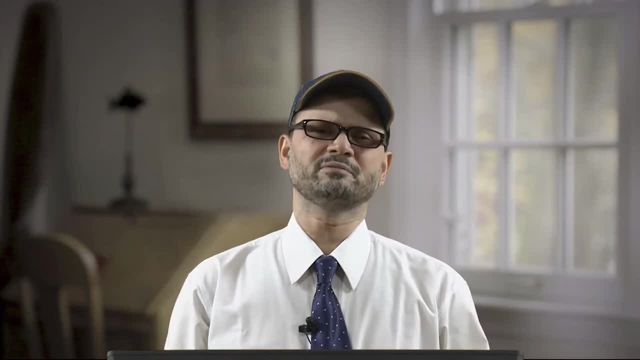 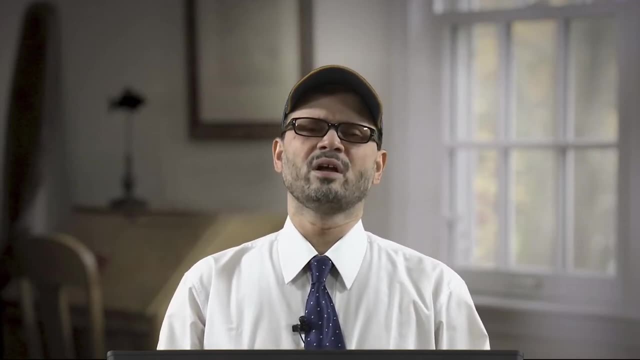 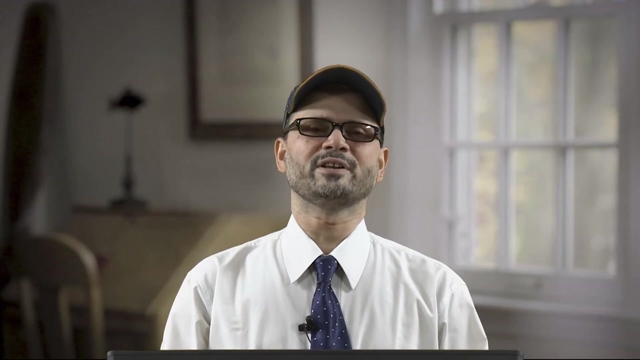 challenge to melt them. So you need a typically larger refractory- you know large, where is been- And heat resistant refractories and, in fact, when you have to make the material from the refractory type of materials, in those cases when they are very, very, you know, having high. 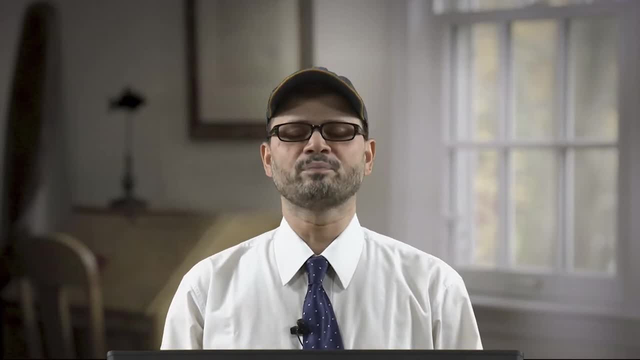 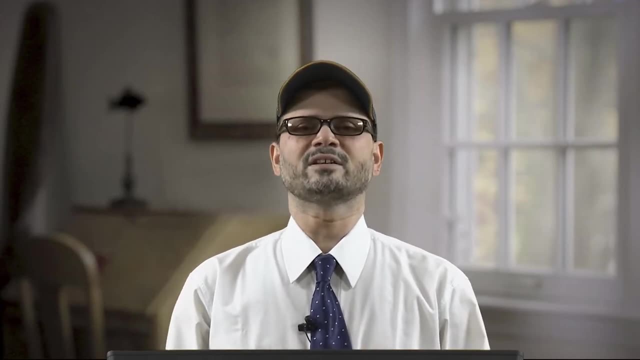 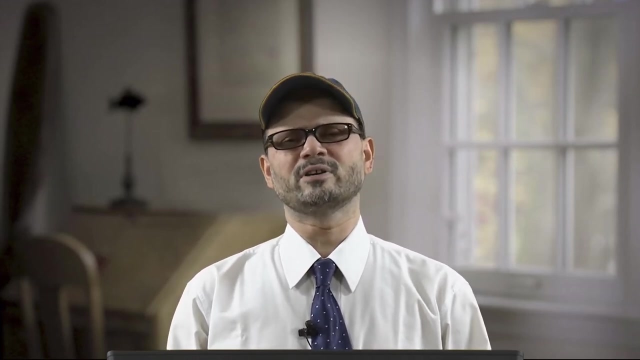 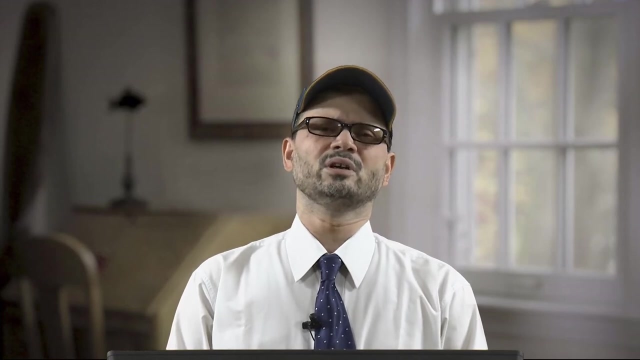 melting point and also sometimes you cannot do by forming, because while forming they, if they, are extremely brittle, So in that case you cannot do by forming. So basically, what we have studied, that what we know about the different type of manufacturing methods, like casting, but in casting you have limitation of the melting point, So when the melting 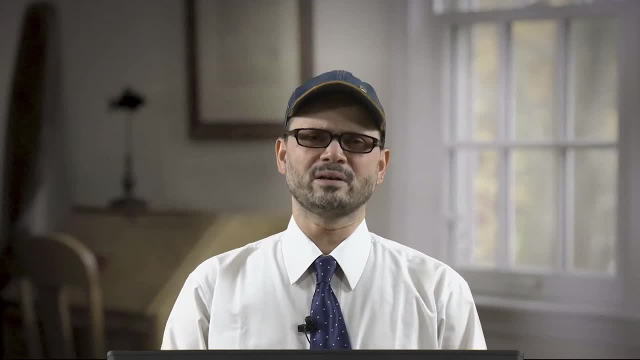 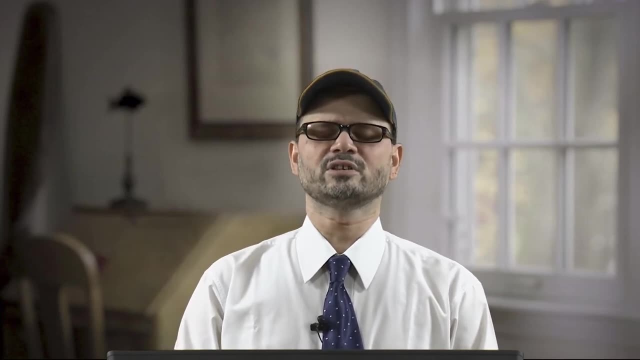 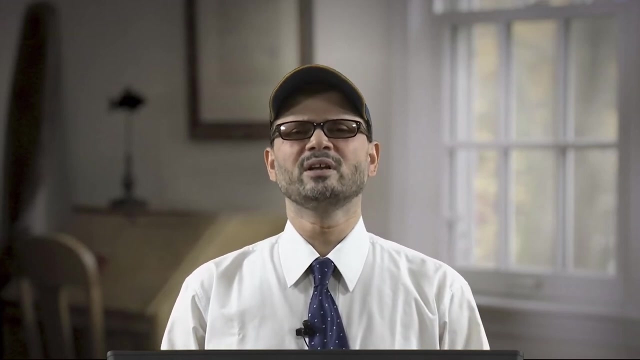 point is extremely high. in that case that limits the castability behaviour of the- you know, material caste ability of the material similarly forming. So when the material is not at all ductile, even at higher temperatures, it is not sufficiently ductile to be formed into certain shape. in that case you cannot do by forming for melting. 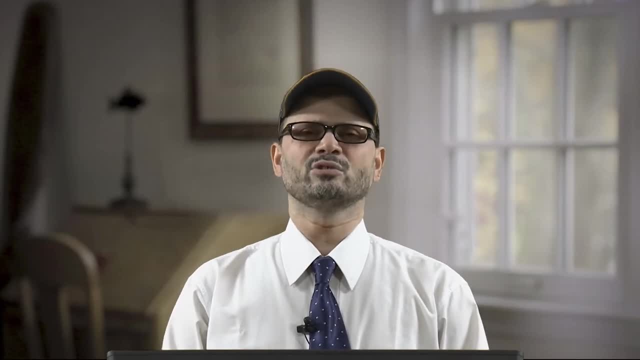 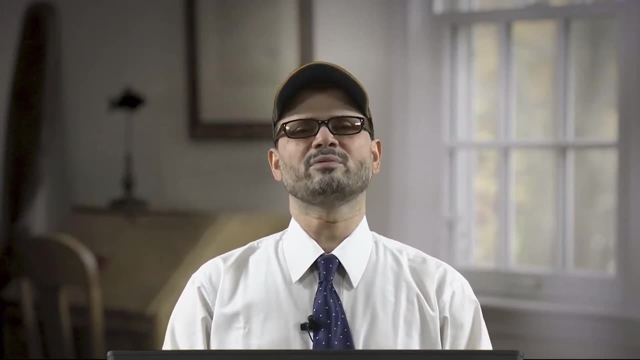 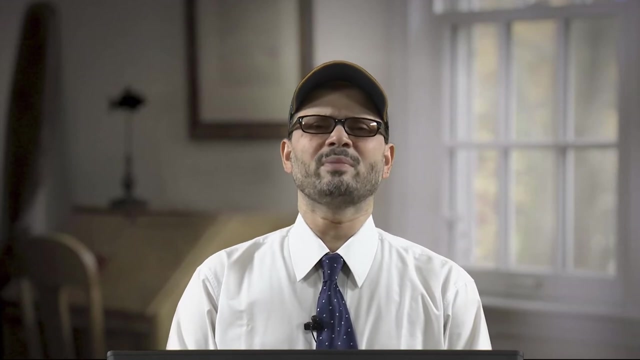 also a material of, as you know, not very high melting point. So that way weldability may also be affected because of many properties, may be because of its conductivity, because of its other properties. So when all these type of you know manufacturing methods raise their hands, they are not you. 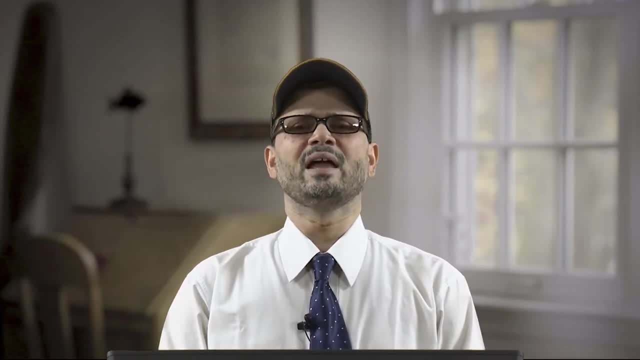 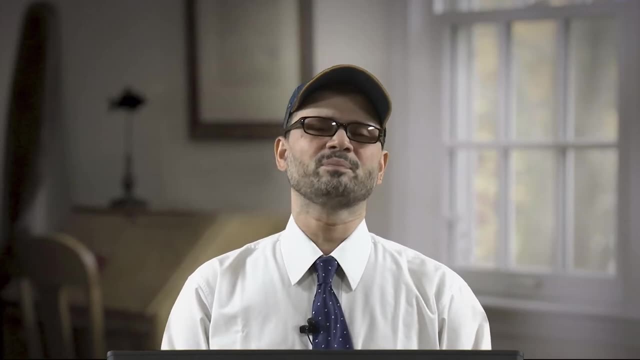 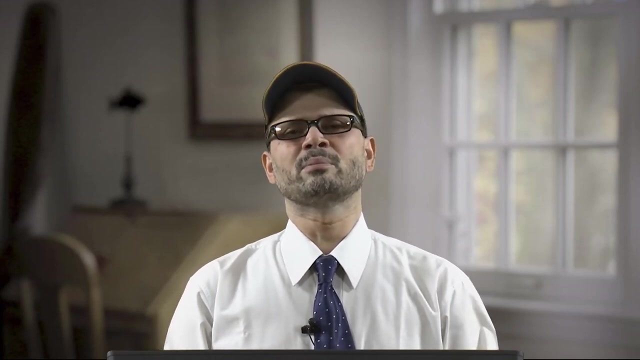 know suitable for making a material and in the material you require that type of you know, and when you have to design some cast product, some product, basically, where you need to induce these elements which have, which is expected to produce some specific type of you know, properties, In those cases you need to use this powder metallurgy route, and that is why this powder metallurgy is quite important. Then you have the wastes very, very little, And so powder metallurgy processes. wastes are very, very little material. about 97 percent of the starting powders are converted to products. 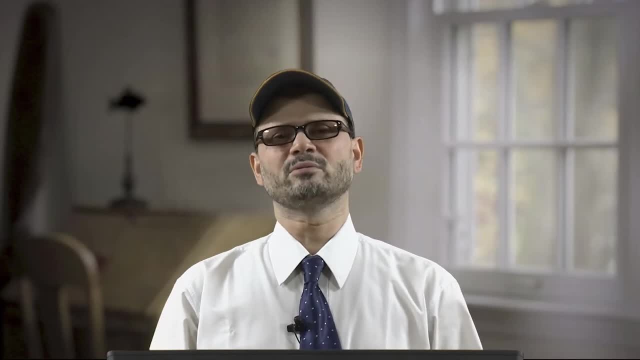 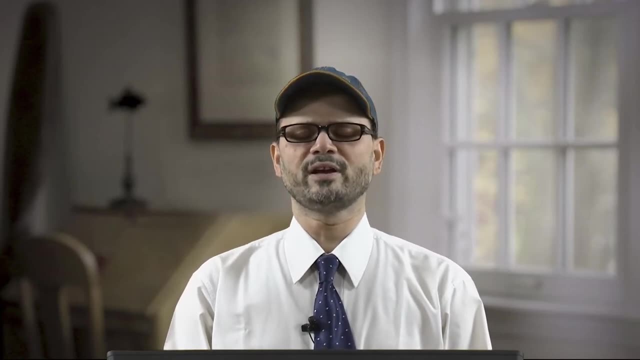 So you do not have to worry about the productivity of the process. you have very less wastage of the material. Then powder metallurgy parts can be made with a specific level of porosity to produce porous metal parts. This is another advantage of the material. 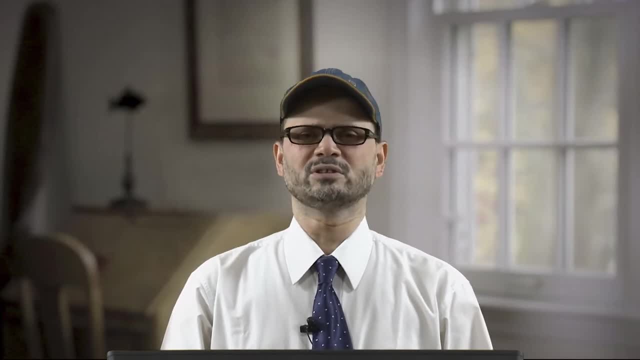 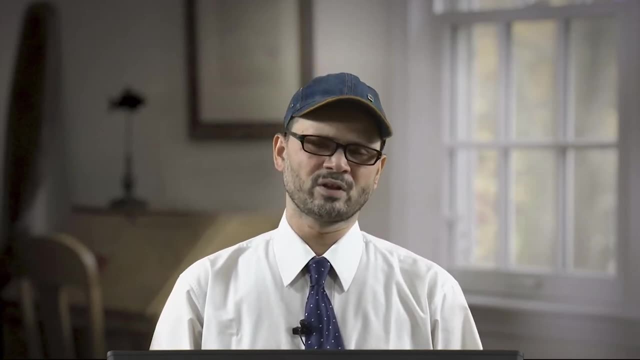 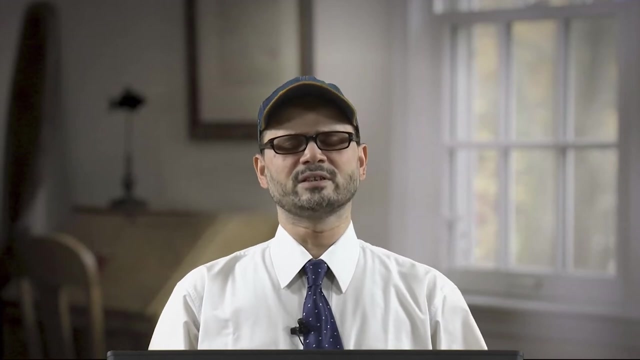 So this is another advantage of the material. So this is another advantage of the material- Powder metallurgy- because you cannot very easily make the products with specific porosities when you have to control the porosities. So those things can be made only by powder metallurgy, because you will certainly get. 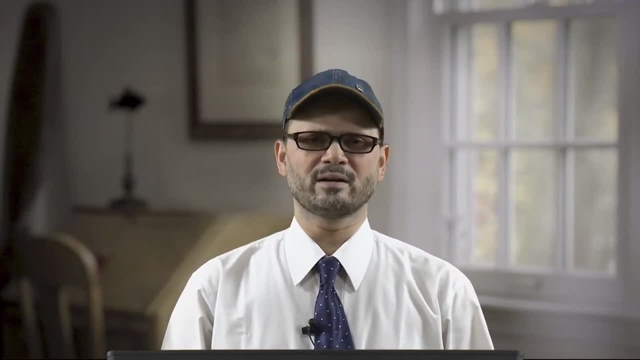 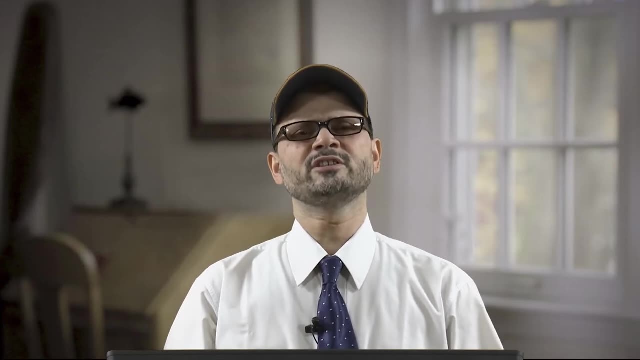 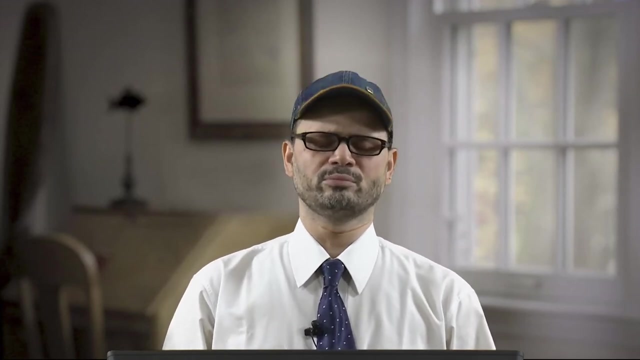 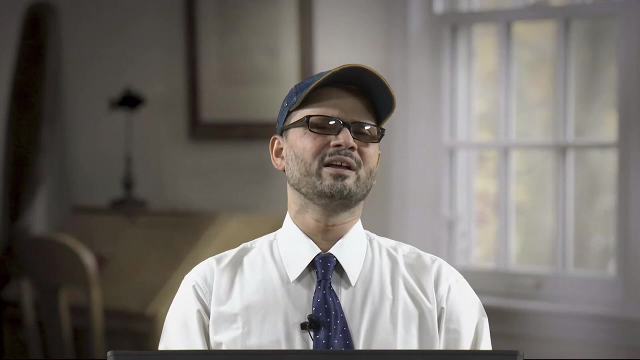 certain level of porosity in casting cast products and when we form it, then certainly we know that the porosity decreases as we form the material, But you do not know the porosity. where it will you know be happening and up to what extent the porosity will be there and then, and that uniform porosity cannot be maintained. 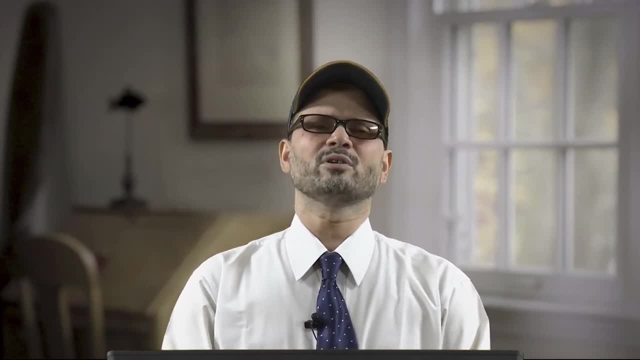 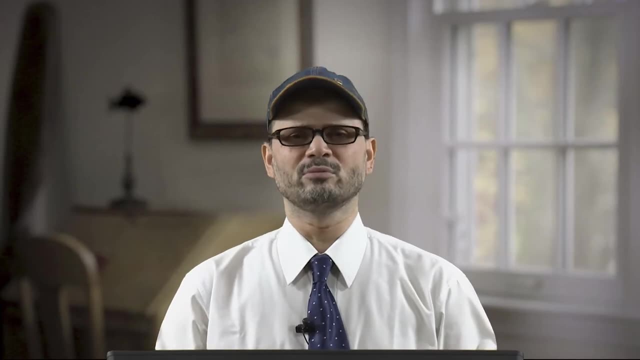 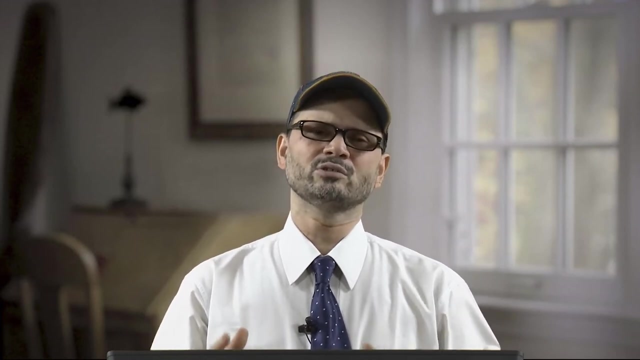 you cannot predict in the case of casting processes. But when you have to have the product with specific level of porosity, and that also should be uniform throughout the domain, then that can be made by this powder metallurgy route, because when you are using the powders then powders are, you know, powders when they are. 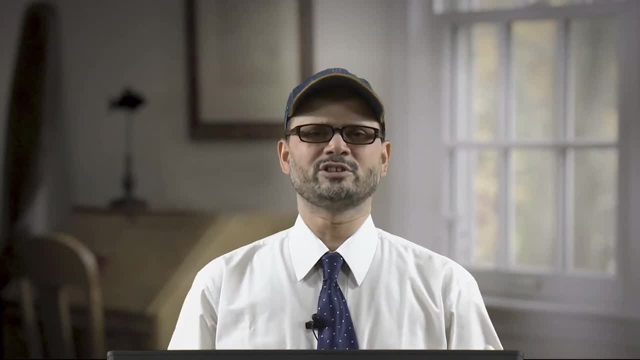 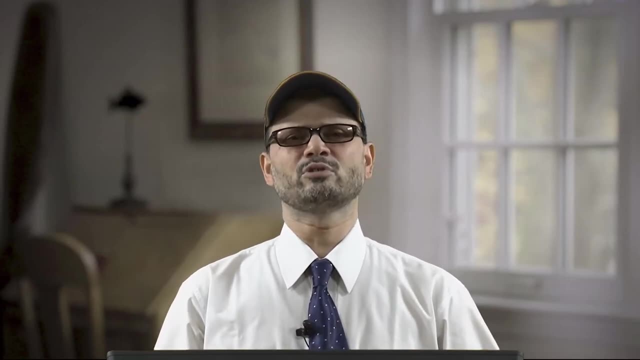 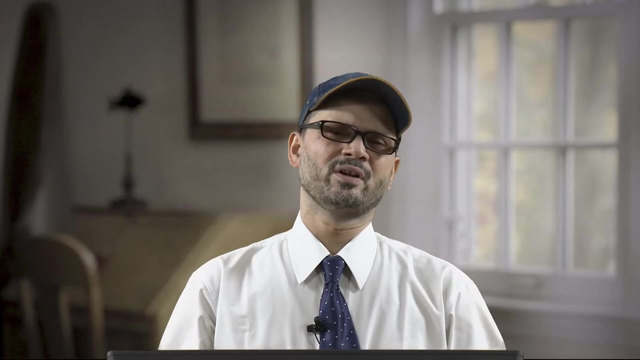 loose powders. you know that there will be porosity in between them, there will be void spaces between them And with degree of compaction, basically the, that porosity decreases and ideally, when the compaction will be quite high. as you increase the compaction at one a level will come when 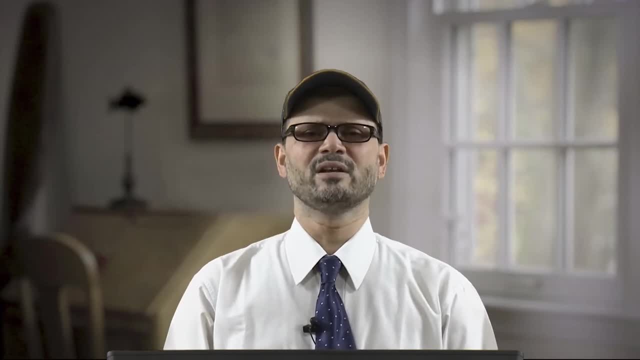 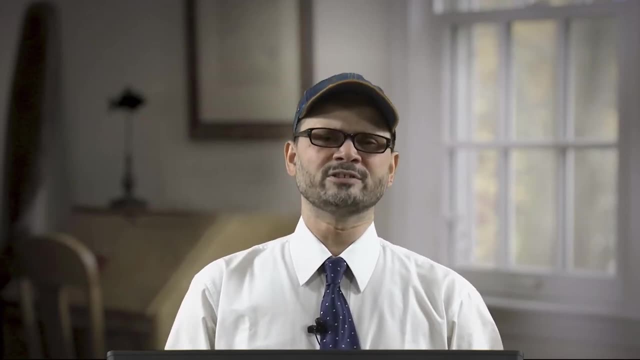 the density will be same as the efficiency. So the actual density of the material, in that case porosity, is 0, but before that, if you treat the material, if you make the material from there, then porosity remains and you can have the material with certain degree of porosity. 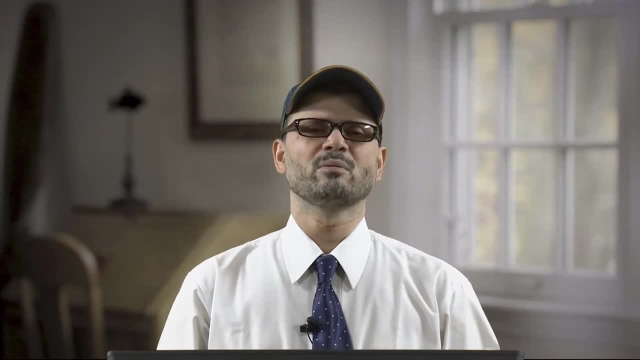 So that is how you can maintain the porosity mostly used in case of bearing applications or so. So this is the only route by which you can make the materials with you know requisite degree of porosity. So this is the you know. 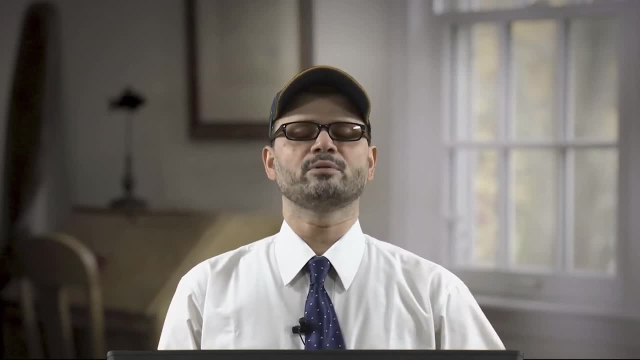 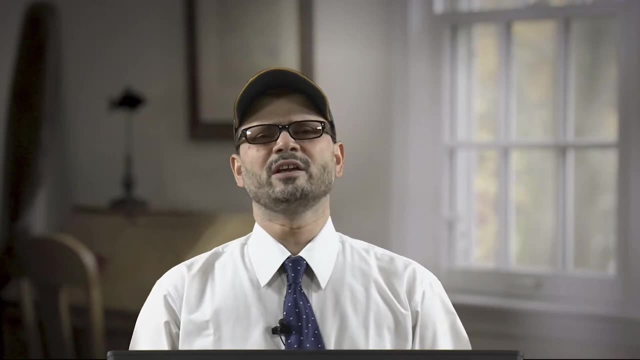 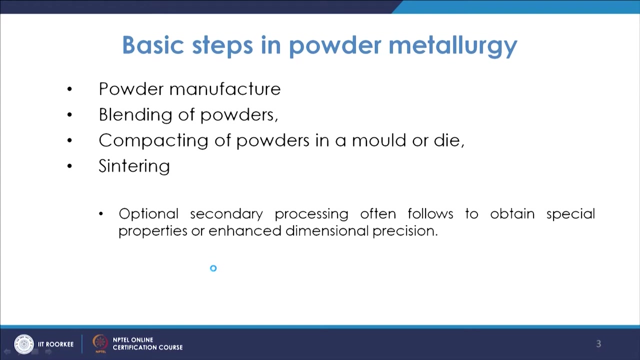 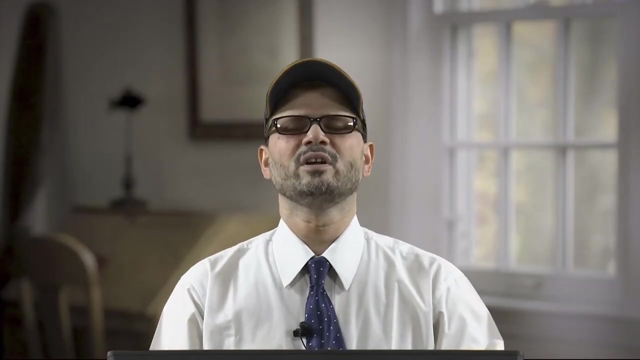 You know trait of the powder metallurgy process: What are the steps in the powder metallurgy? So, as we discussed that in powder metallurgy we use the powders. So first of all we require powders. So powder manufacturing is important. you have many methods of powder manufacturing. 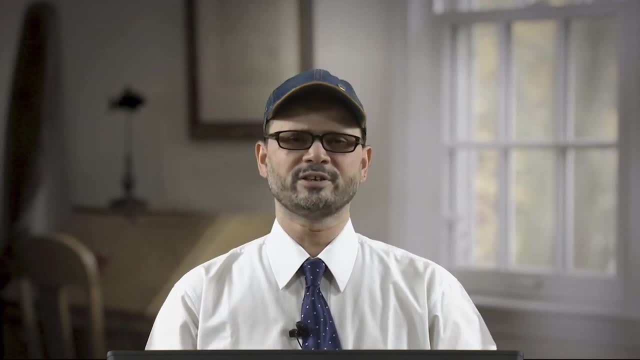 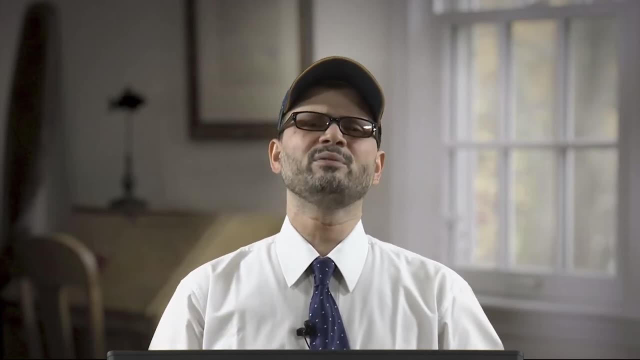 you require, basically, powders of high purity. You should do, You should do. You should not have the impurities with the powders because if they have they are impure, they are going to be with the powders inside the when you are going to further. you know. 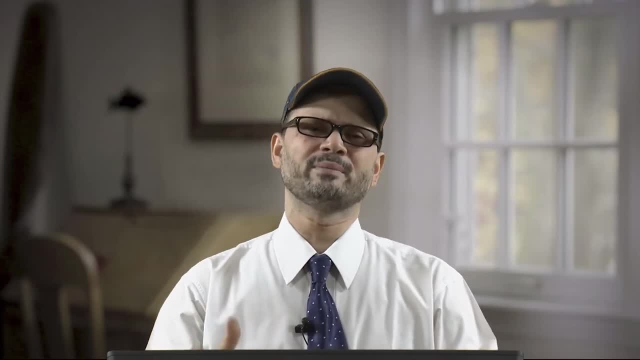 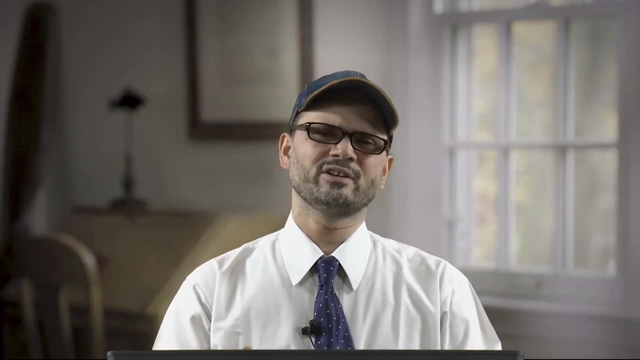 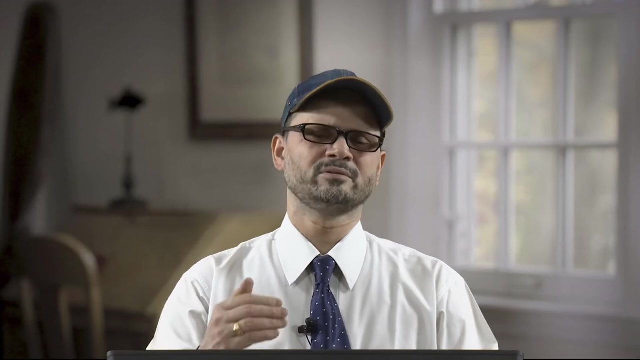 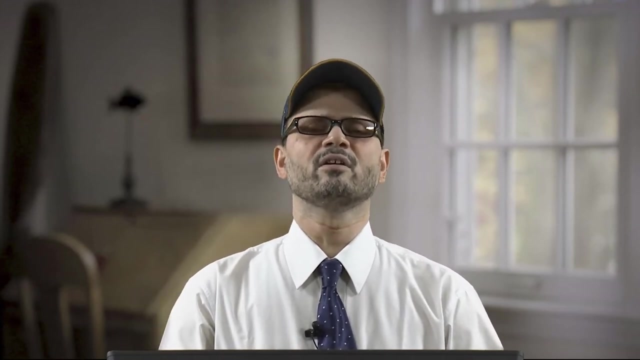 treat them. So you require, you must use many methods you use. we will discuss about those methods. So methods are used to generate powders, to make powders of different materials and then use them or treat them further. So once you have powders, then you require the blending of powders. 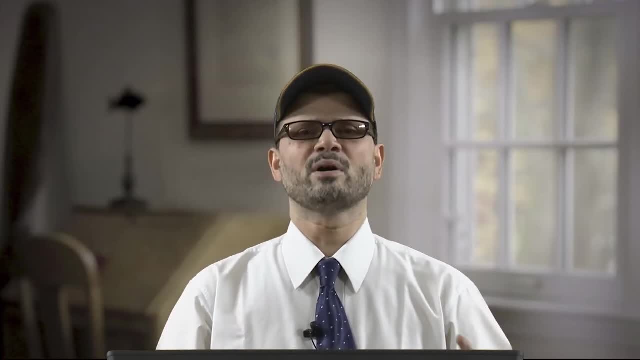 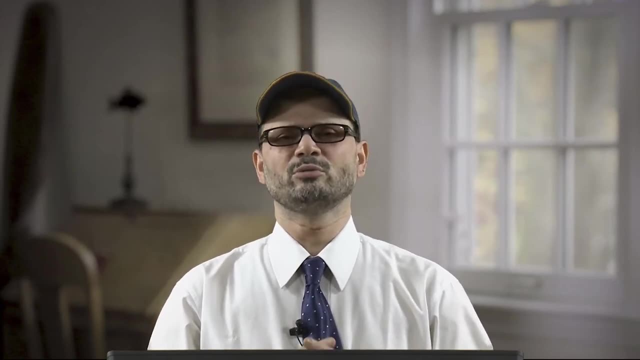 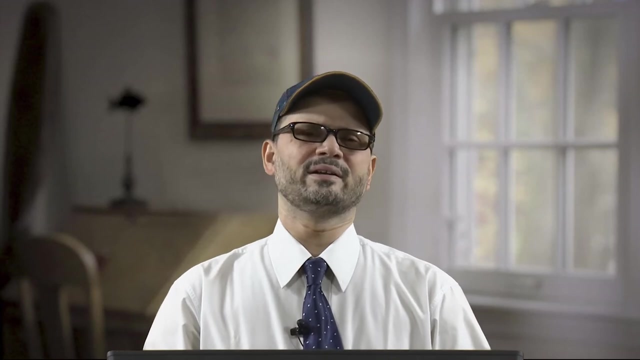 So blending of powders means you have to mix the powders you know as in proportion desired. So blending of powders means they should be uniformly mixed. you should have the technology to mix them properly and then for blending you require certain medium. also, you may have 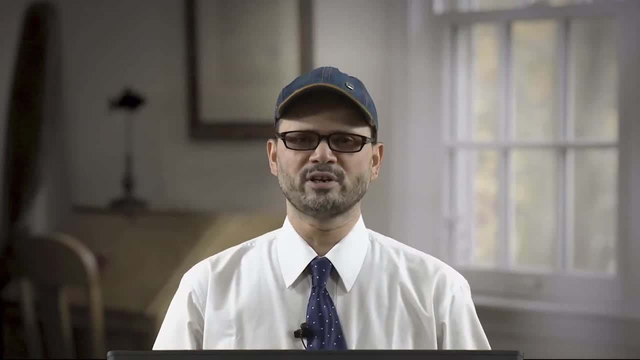 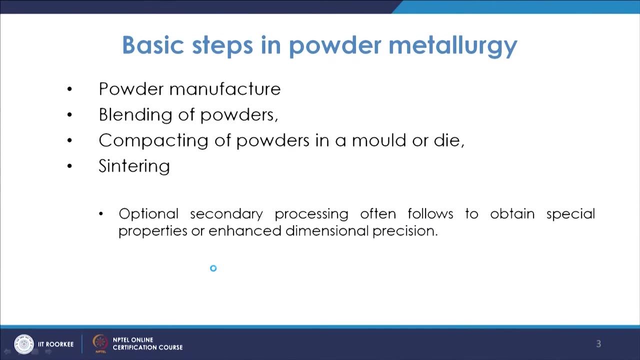 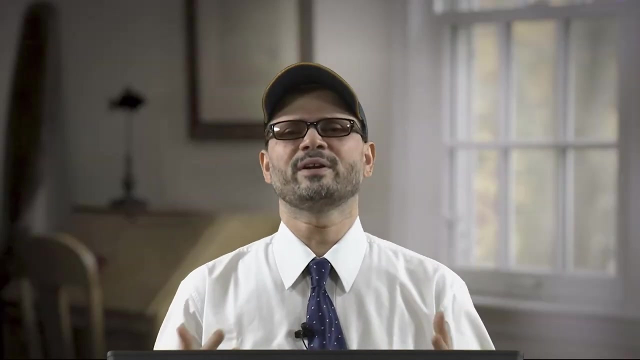 the binders, So which is required to blend them properly, so that blending is very much required. Then, after blending, you require the compacting of powders in a mold or a die. So once we mix the powders of different materials, of different composition, then next is to make. 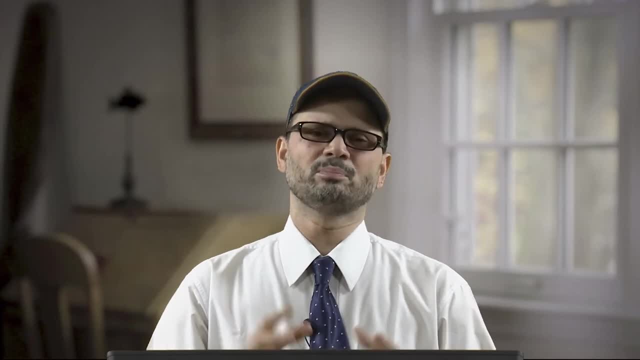 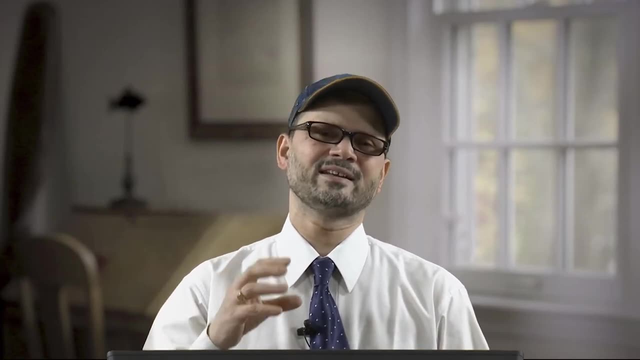 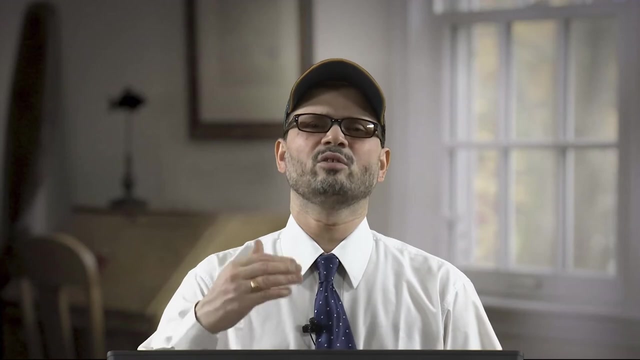 the compaction of the powders. So the powders are compacted in a mold or die under pressure, And when they are compacted and given a shape and the moisture is still there or binder is still present in the liquid form, then they are known as green compact. 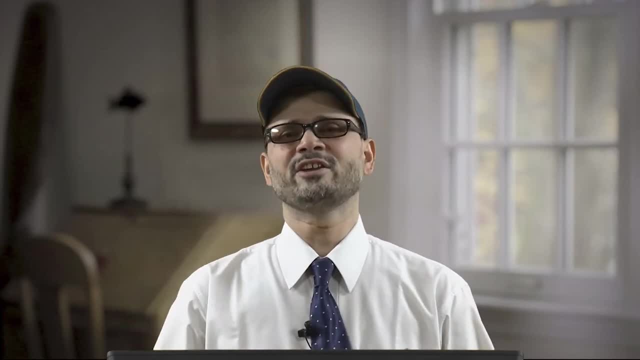 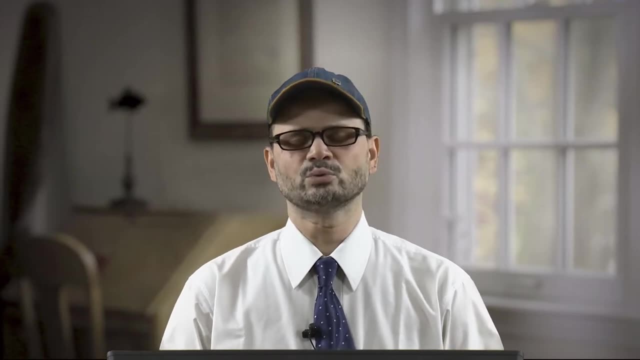 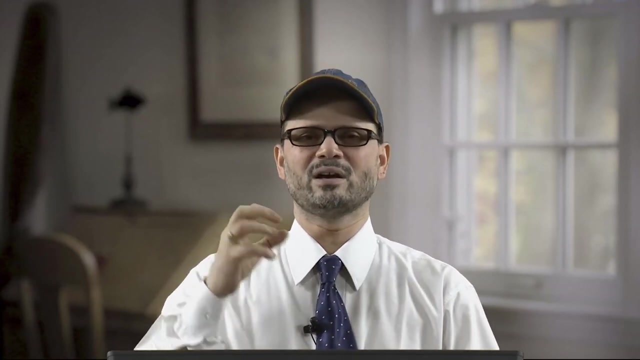 So, first of all, just like we make the green sand mold, So similarly you have the green compact formation, initially when we have the binders into the- you know- powders mixed with the powders and then blended, And then you are having 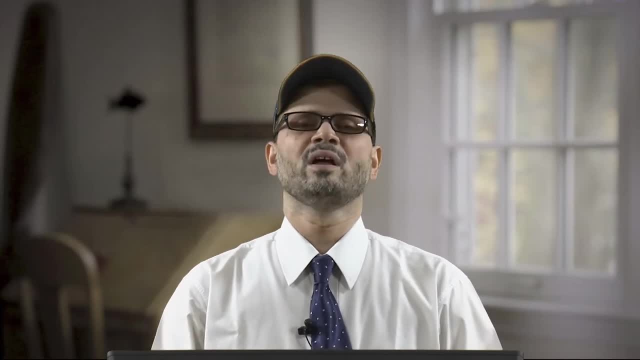 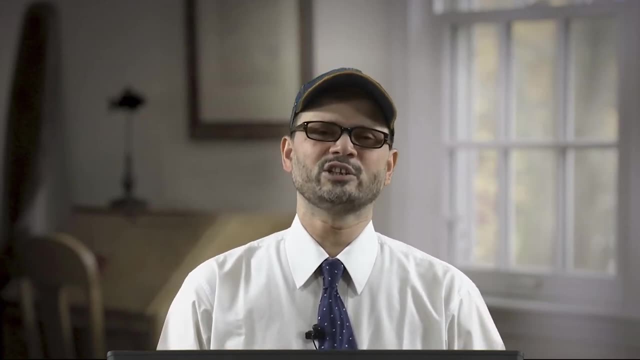 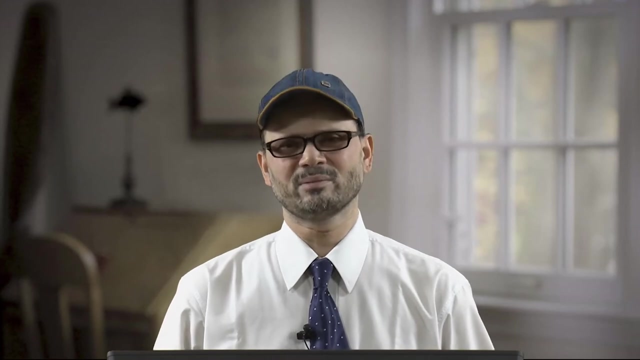 putting them in a mold or a die or in a press, and then you are making a compact of the powders. Now, compaction is done basically to reduce the space between the particles, as we know that when we have loose powders there is enough space between the powders. the density is quite 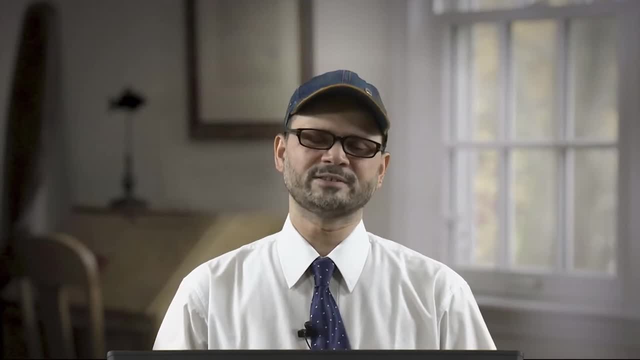 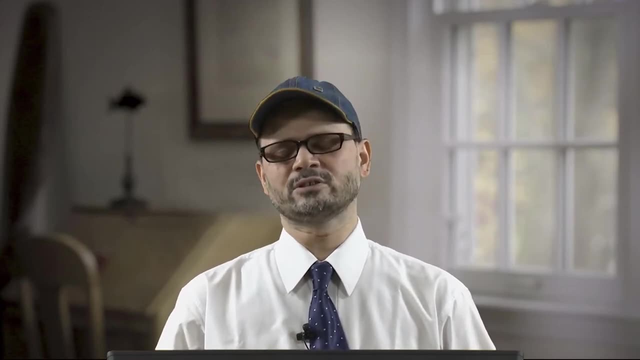 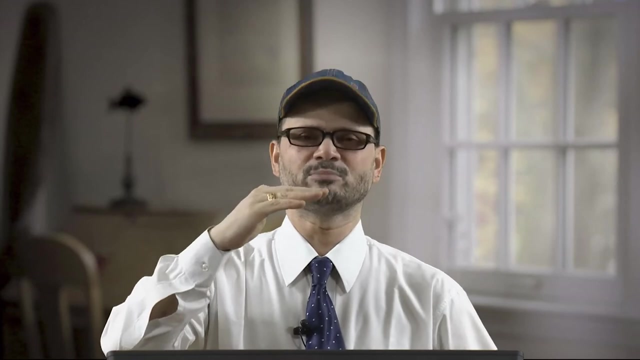 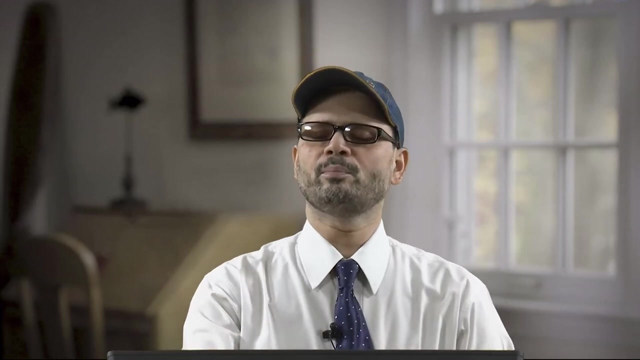 less, but then once we start compacting, then they come closer and closer and you have many methods of compaction. basically, you can compact from the top. you can compact from top as well as bottom, So as we know that when we have a surface and you know when we compact, so basically, 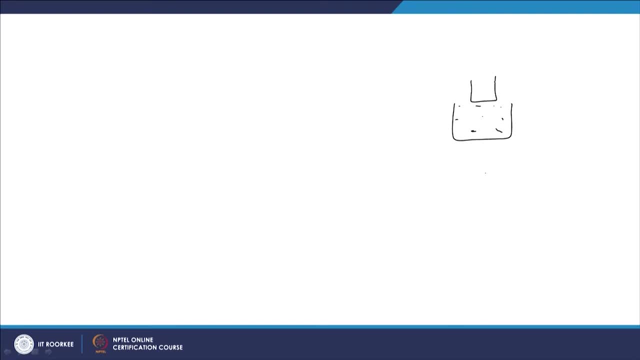 when you have the powders and if you are compacting from here. So this you know material, this you know powder, which is there of this shape So slowly, So that may come to this shape. so this will be coming to this smaller dimension. 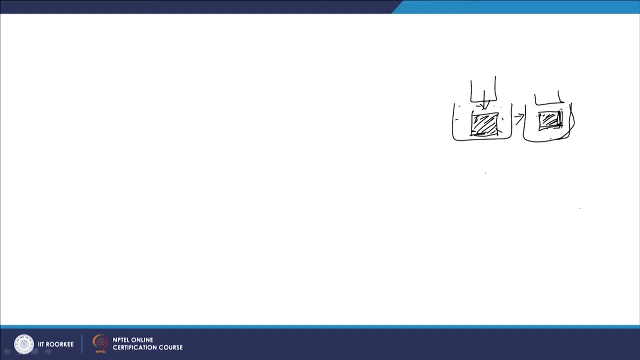 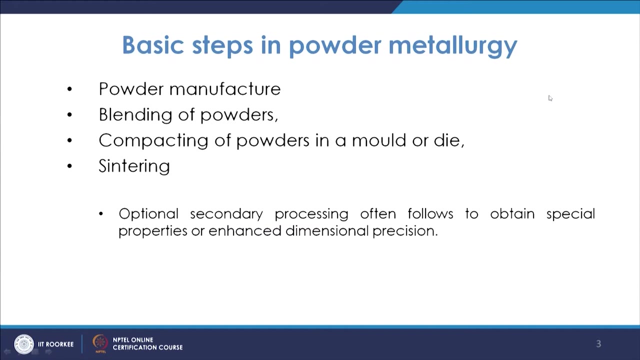 So this lateral dimension will be same, but this height will be reduced. So this will be going to this dimension. Now the thing is that when we do the compaction from the top, then that case your compaction density will be decreasing as you go down. 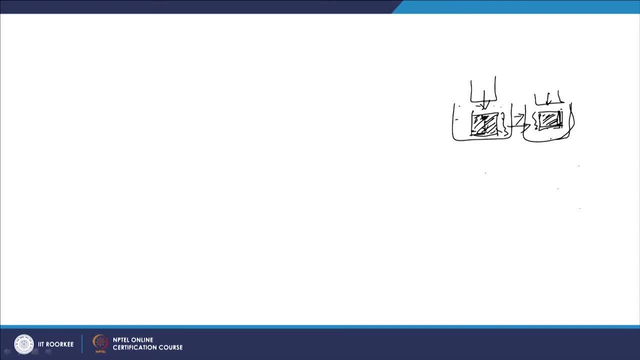 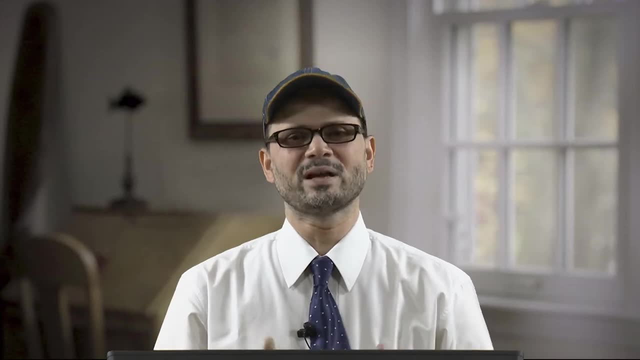 So maximum compaction will be here and as we go down the compaction density is so density will be decreasing. So compaction methods are also important how we do the compaction. we have to do from one side, single acting, or we have to double acting compaction. 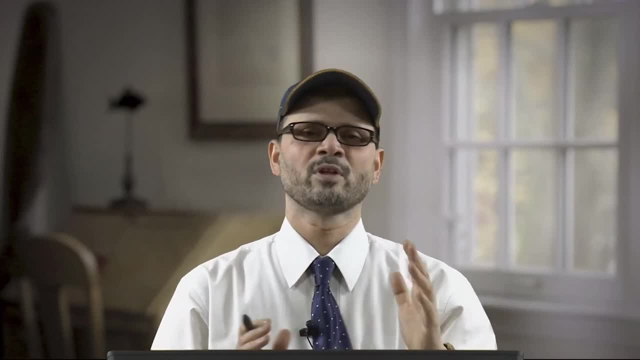 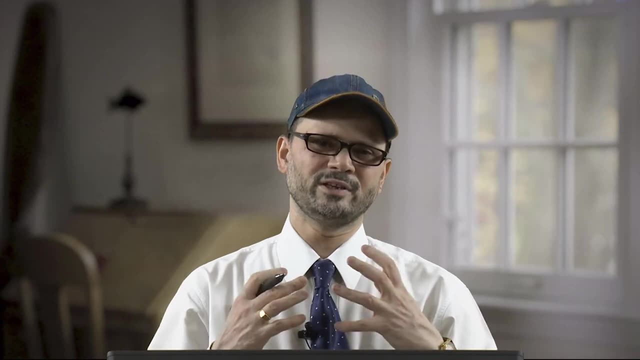 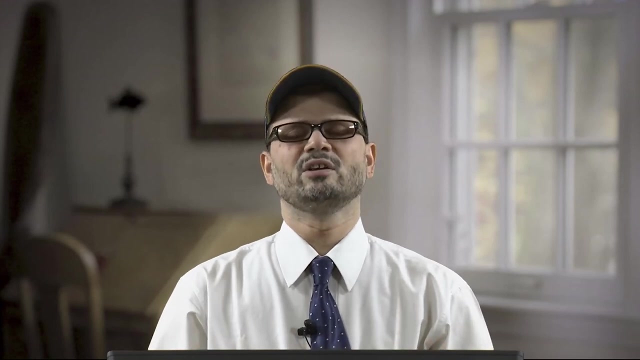 So that compaction is very important to have the proper compactness among the powder particles because that will be, you know, talking about, or that will be represented. So that will be representing basically the density of the parts in the various, you know, places of the component. 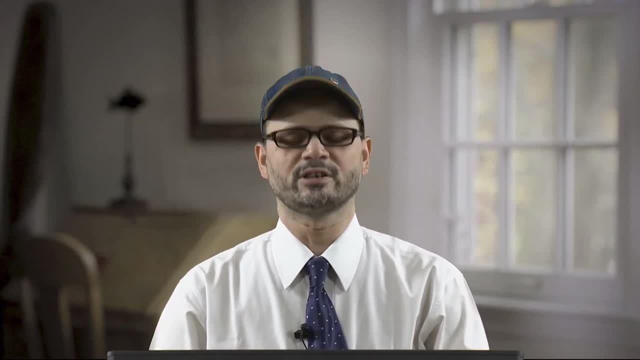 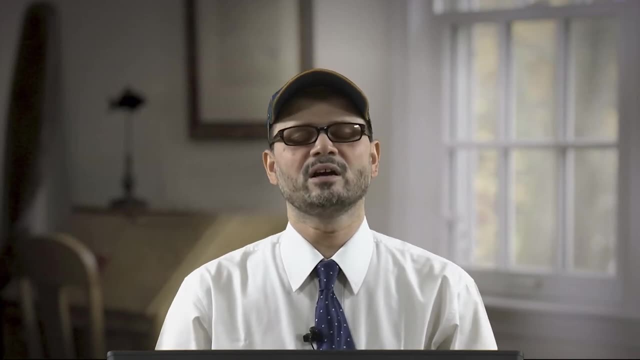 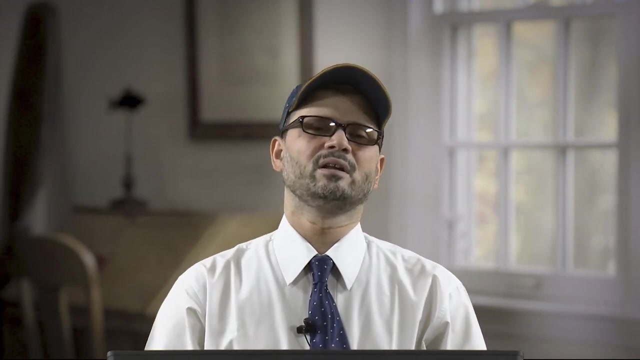 Then the important stage is sintering. Now sintering is done. basically sintering is done in stages, but the sintering is important in the sense that when we are compacting the material, then still when you have the green compact. 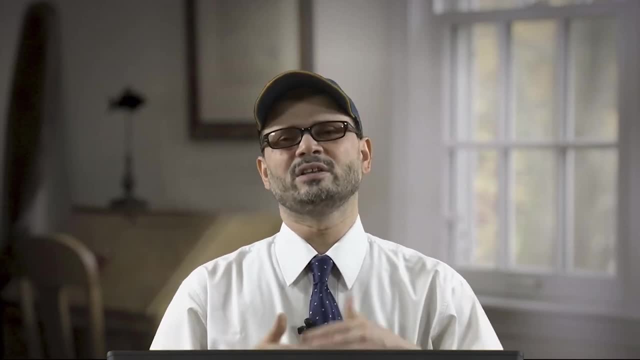 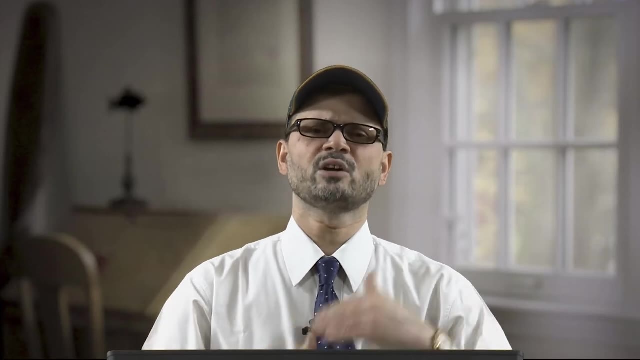 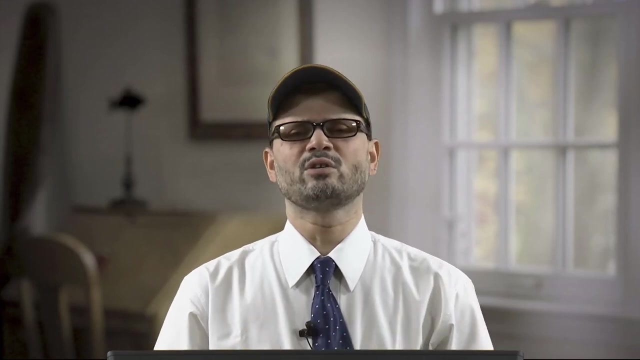 Then you have the presence of moisture or the you know lubricant is there also Now this. you have volatile- you know materials into it. Now they need to be driven off and in fact you know that is. it is also required to have the strength. now you have to increase the strength, so you have to increase the bounding. 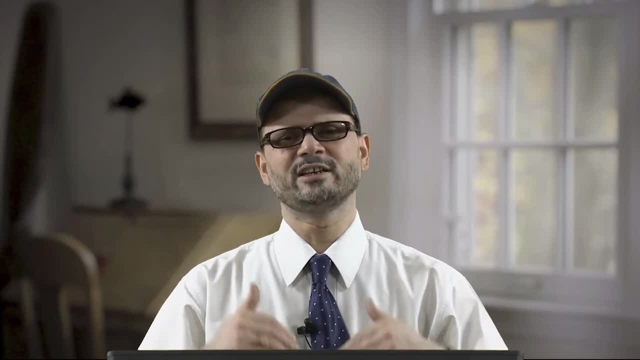 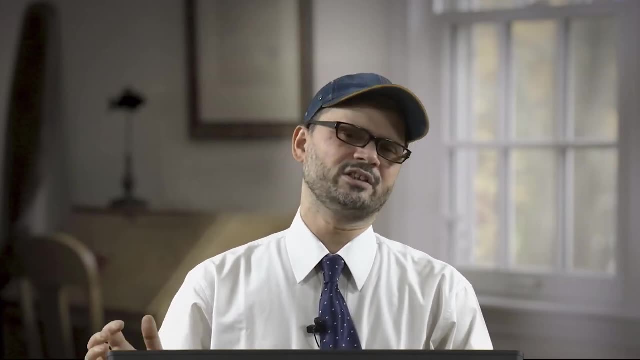 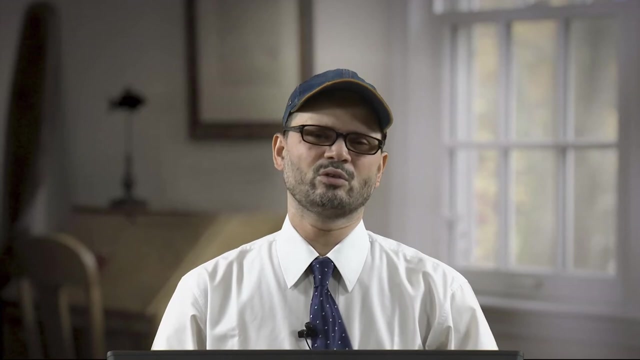 So what it does is before the melting point, so it is heated below the melting point of the material And in that process, basically initially you have, So you have different stages in which basically the all these volatile materials, they are going away, then wounding develops and then you get basically a material with quite good strength. So that is your sintering stage, Then optional secondary processing and after that there may be secondary processing requirement, which you know is required for the enhanced dimensional precision. So you may go for other secondary precision or secondary processing to achieve the desired. 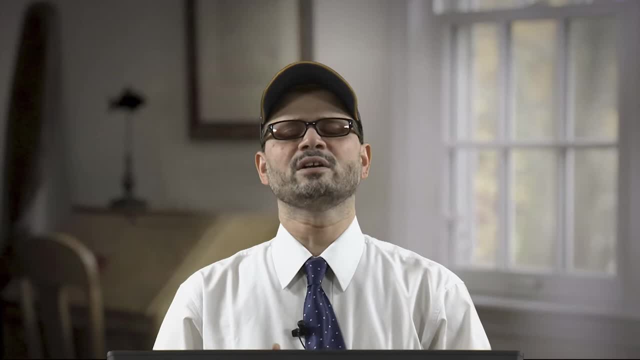 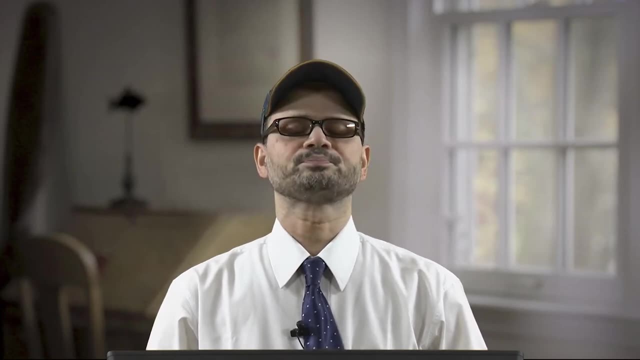 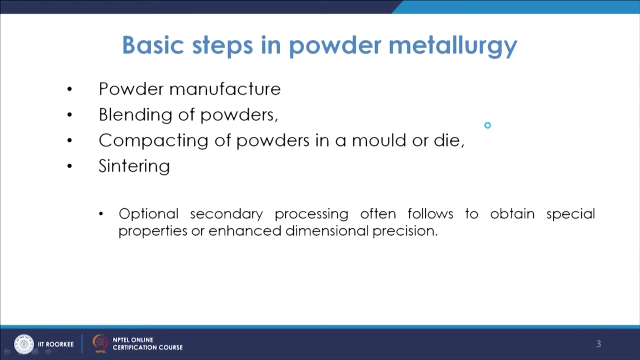 type of properties in the material. So that is what the different steps are there in powder metallurgy. you know products. So first of all, as you are discussing that, you have powder manufacture and for powder manufacturing you have different methods, and we will discuss about the different methods. 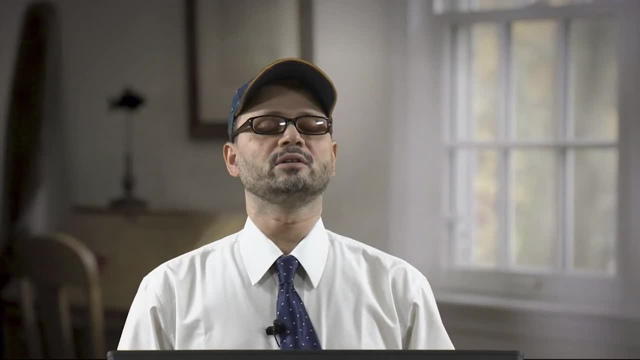 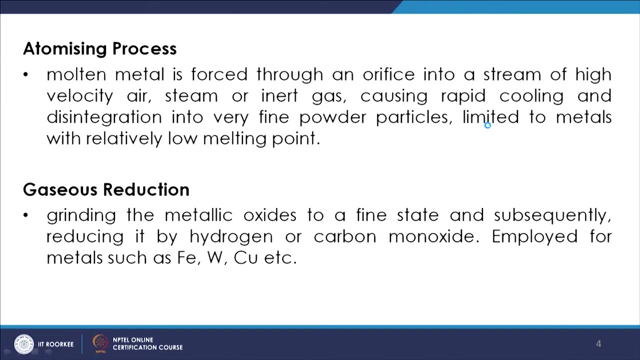 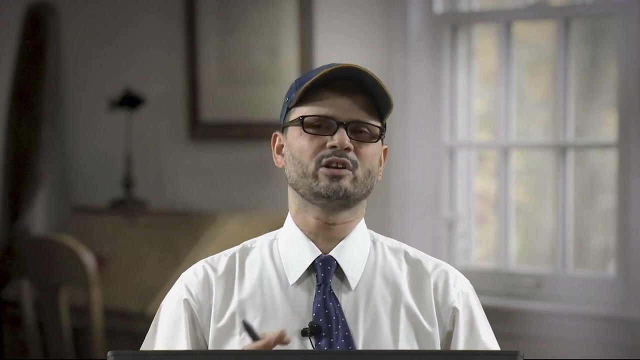 of powder manufacturing. So the first process which is there for the production of powders is the atomizing process. So in the atomizing process, basically, you have the spray of the material At in atomized form. so molten metal is forced through an orifice into a stream of high velocity. 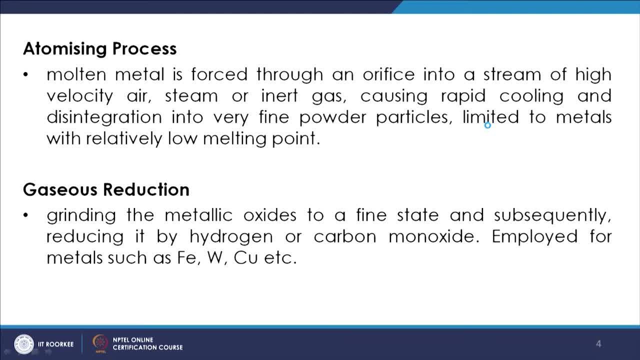 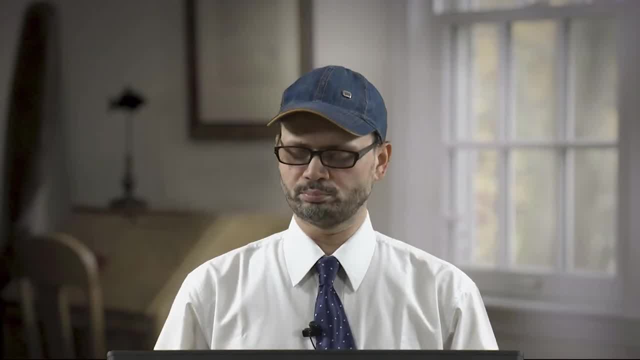 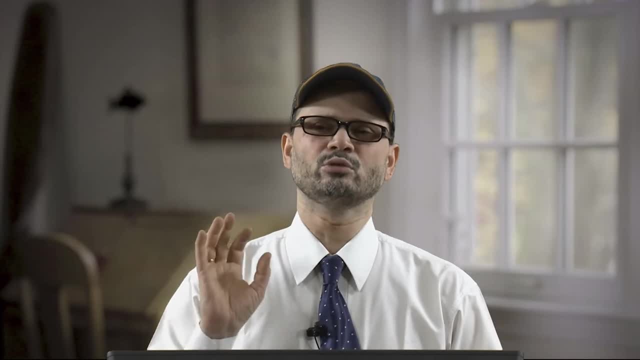 air stream or inert gas, causing rapid cooling and disintegration into very fine powder particles. Now what happens in this case? you produce the fine, you give the fine- atomization of the metallic material. So, basically, you have to have some means by which the atomization of material, 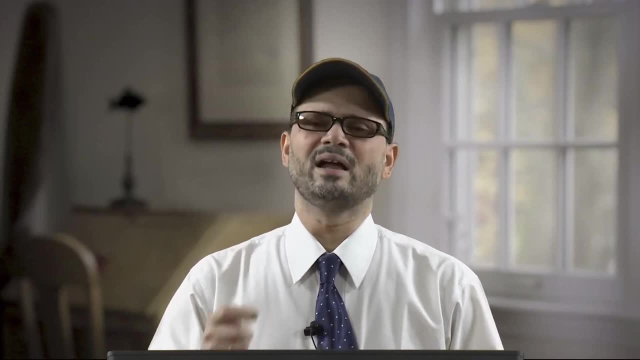 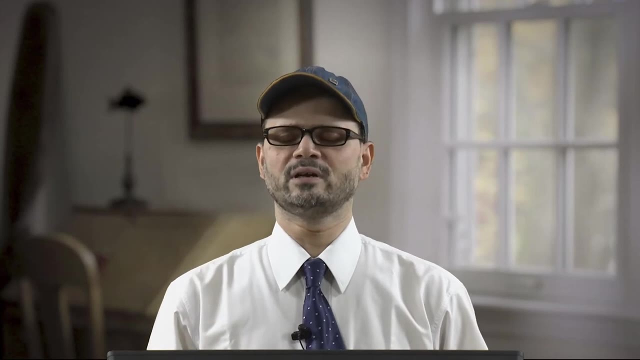 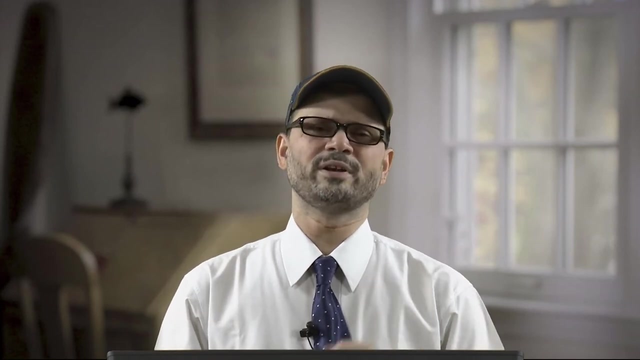 The, you know metal is done and they are sprayed through certain type of nozzle and once they are coming, then they are will be, you know, rapid cooling of these, you know fine droplets, because they will be, you know, surrounded by the cooler medium and they are large surface. 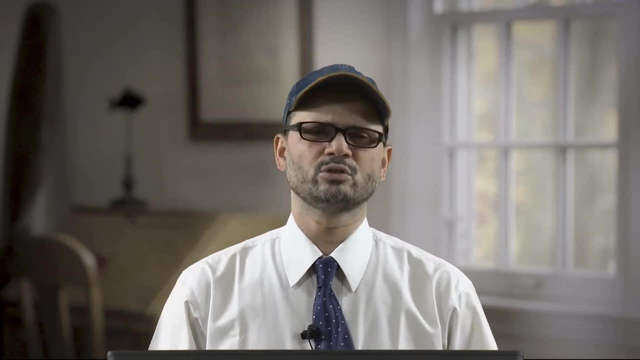 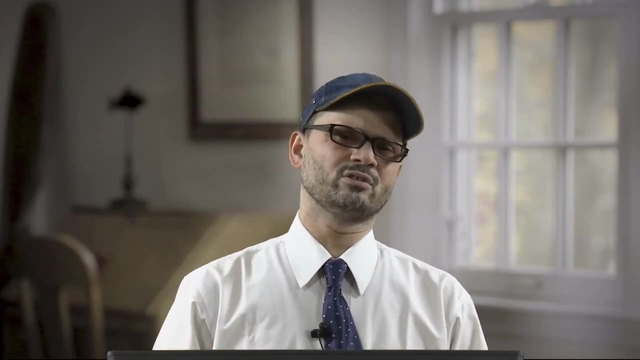 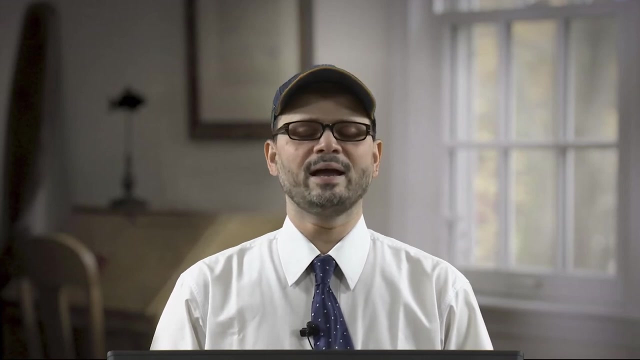 area and they are very, very small volume. So they will be rapidly. you know, they will be subjected to rapid cooling, So rapid solidification, and they will be converted to the tiny droplets of metal. So that is the process of atomizing: atomization, and this is normally limited to the metals. 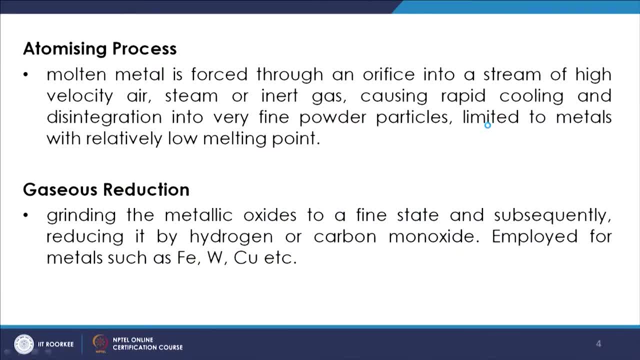 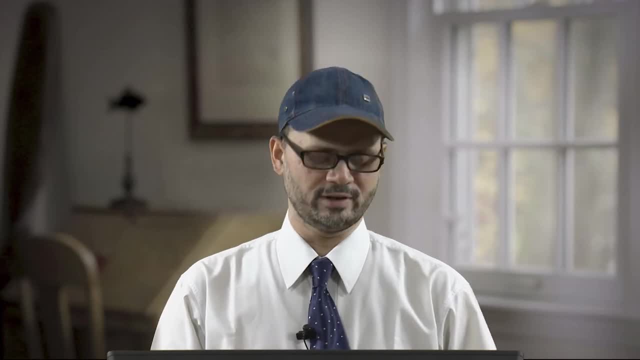 with relatively low melting point. So basically, in this case you have to, basically you know- melt the material. So you require the temperature to be, you know, to be- attained up to that level. So normally we confine it. So we confine it to the metals with very low melting point. 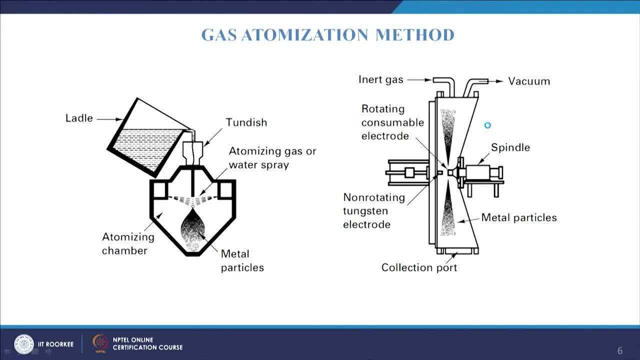 Now, if you try to see the how this atomization is carried out, you can see here that you have. this is the atomizing gas or water spray. So this will be your liquid metal, which will be going through you know a tundish and it. 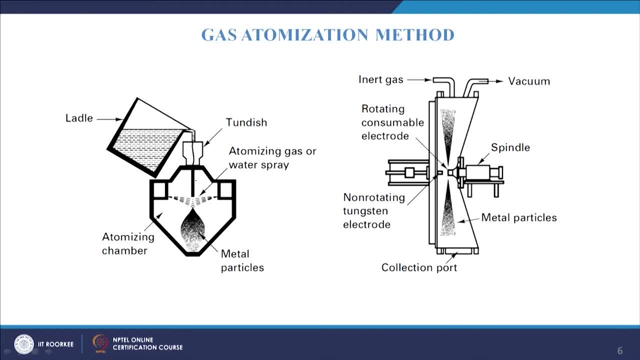 will be coming here and then you are, basically you are atomizing it, And then further you are. So this is a chamber and in this chamber they will be So, since they are atomized, So under the you know whereas, and this chamber is under vacuum. 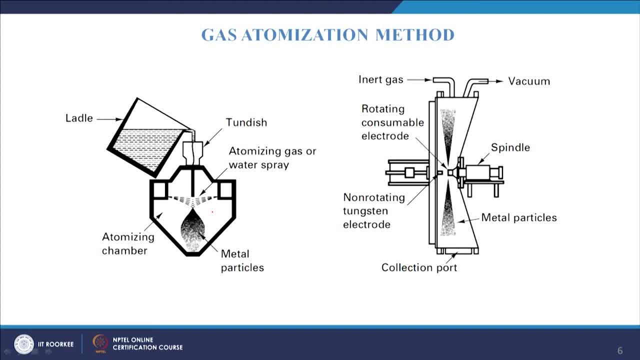 You have inert metal, So it will not be reacting with anything and be getting cooled, So subjected to very high heat transfer rate. So you get the fine metal powders, which is So you go go for this atomizing gas or water spray And because of that it is subjected to sudden 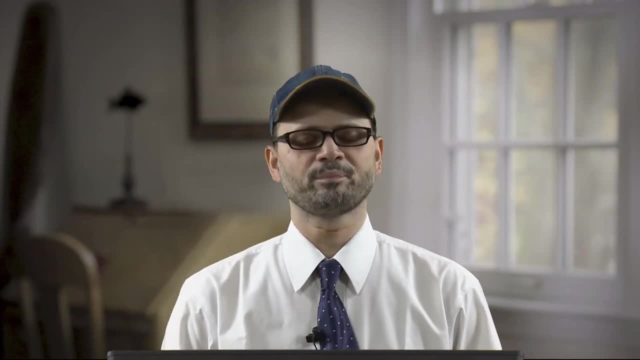 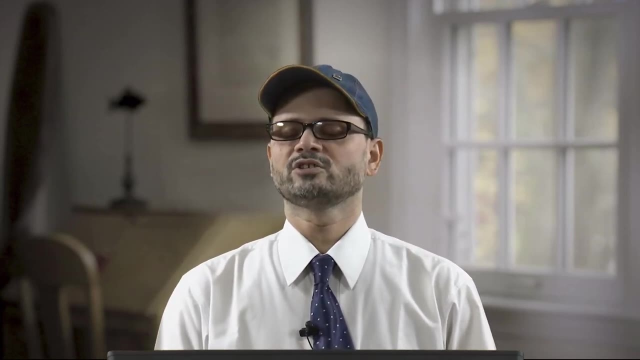 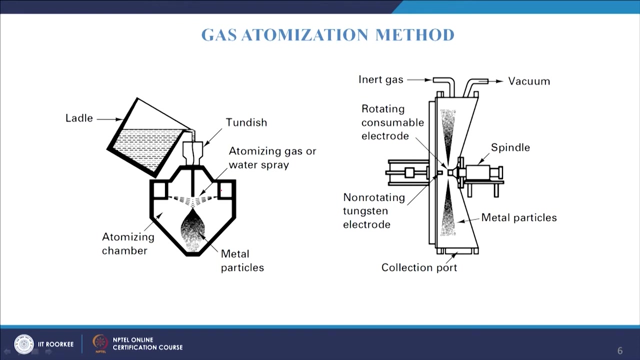 cooling and you have very fine droplets, So they will be converted to very small size of the. you know metal powders. Similarly, you have the. you know gases. So this chamber, you have the. this is the electrode and you know. this way you have the produce. 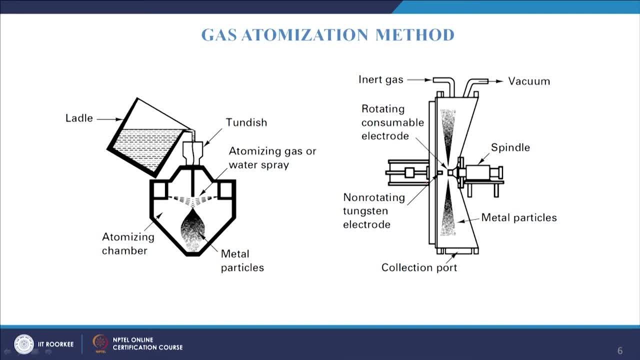 and production of the arc. So, because of the large centrifugal forces, this arc will be going towards the upper side, outer side, And then they will be cooled because of the inert gas is coming through here And then they will be cooled and inert gas is there. 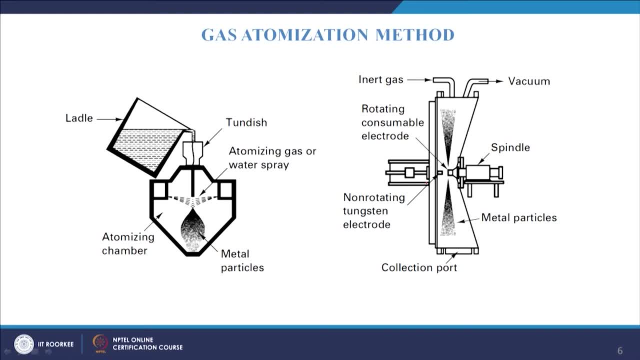 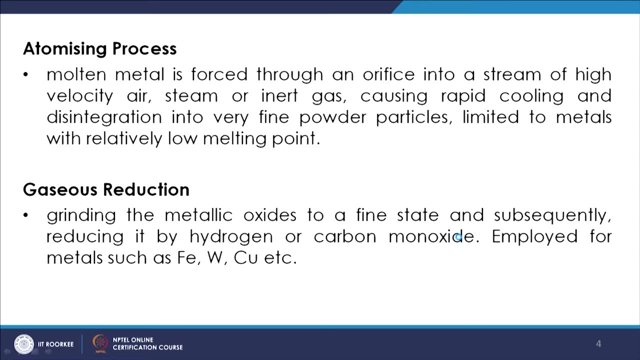 to maintain that atmosphere inside, And then they will be cooled and they will be, you know, solidified and they will be collected at the bottom and they will be taken. So, basically, So, basically, these are the methods by which you get very pure metal powders using this. 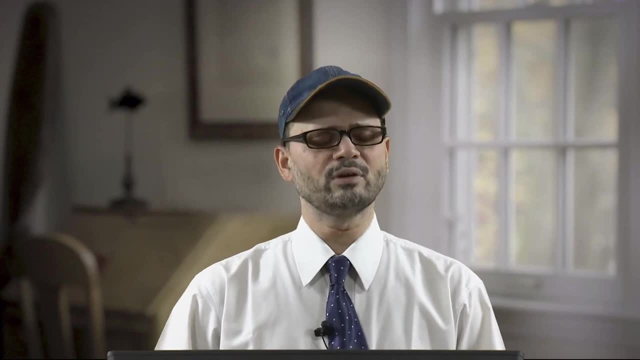 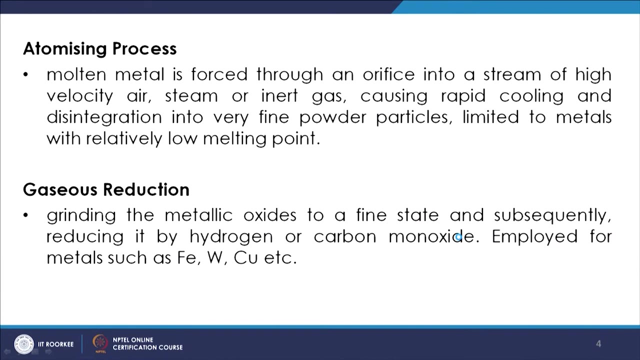 atomization process. Then you have gaseous reduction and in the gaseous reduction process, basically you can grind these metallic oxides to a fine state and subsequently reduce it by hydrogen or carbon monoxide. So many a times you have the availability of the gaseous oxides as compared to the pure. 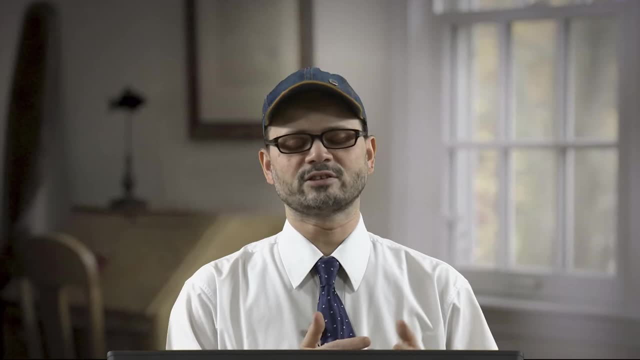 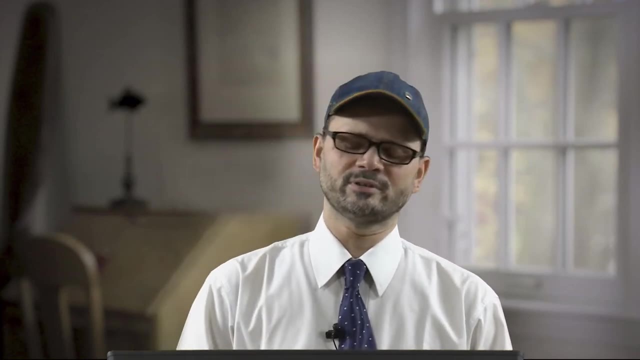 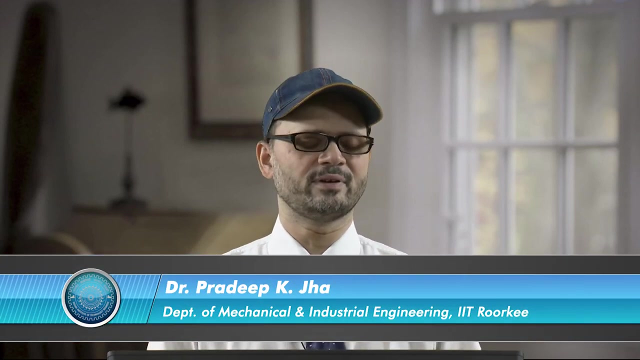 you know metal. So metallic oxides, not gaseous oxides, metallic oxides are abundantly available And in that case you can use these metallic oxides, and you can, you know, I mean crush them to fine state and then further you can reduce it. 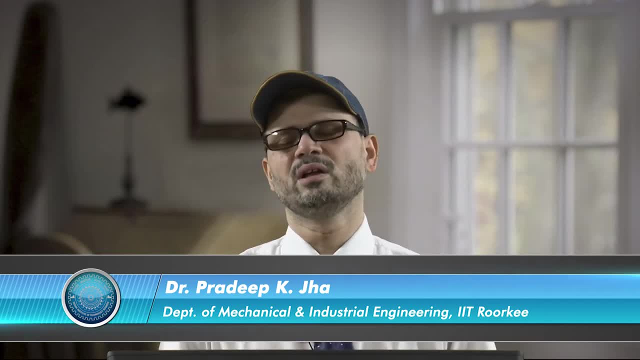 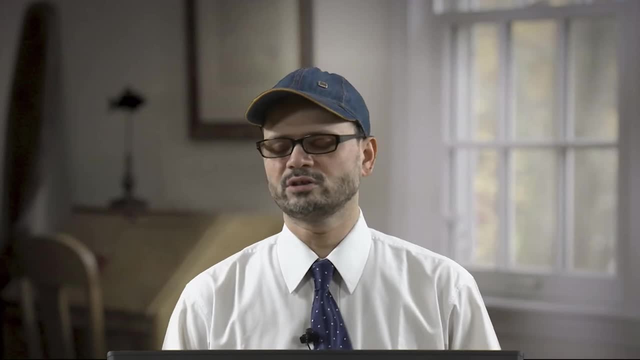 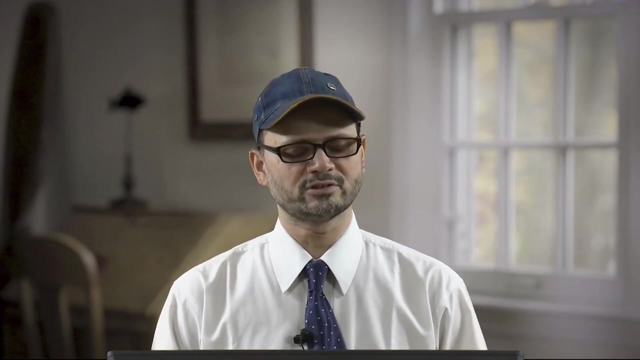 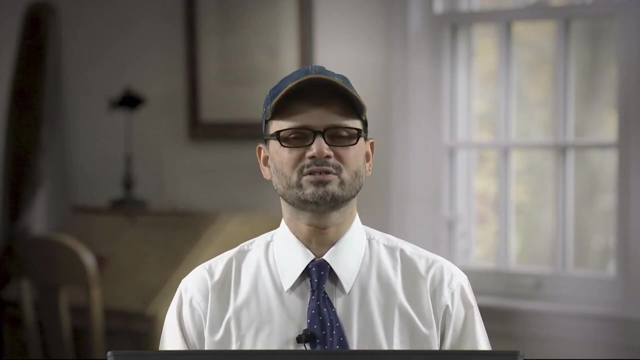 The oxygen part will be removed, leaving the pure metal part, So that way you can get the pure metal powders for the use. So it is normally implied for metal such as iron, tungsten, copper, where the metal is available in the form of its oxides. 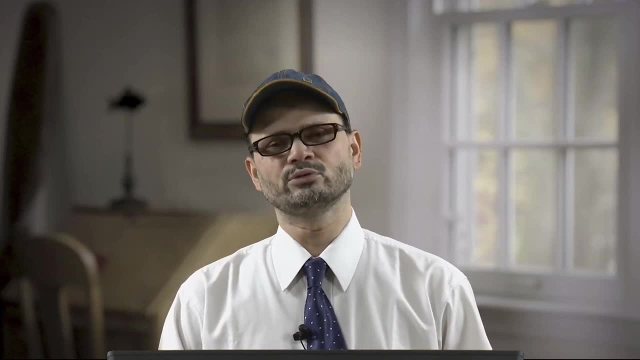 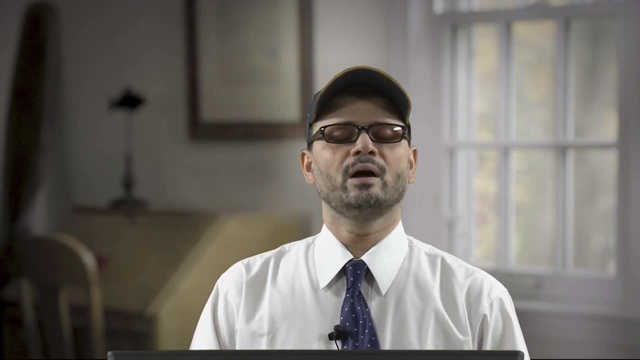 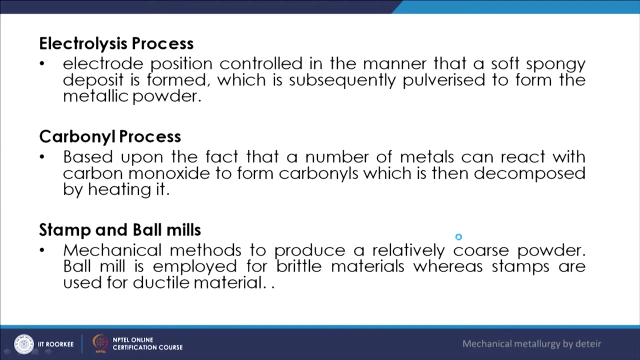 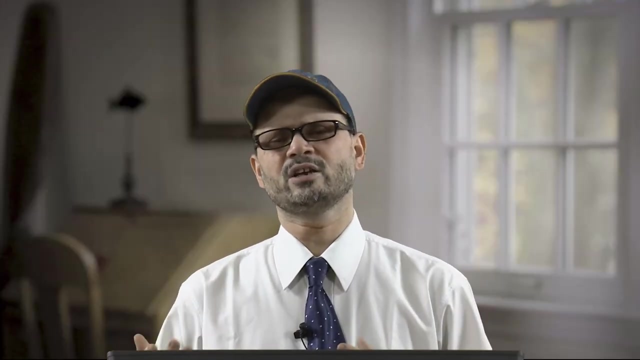 So that oxides can be reduced. to give you that you know pure, you know pure metallic powders. Another you know process is the electrolysis process and you must have the knowledge about this process where, using that electrolysis process, you know that you have two electrodes, cathode and the, and the anode, And you can 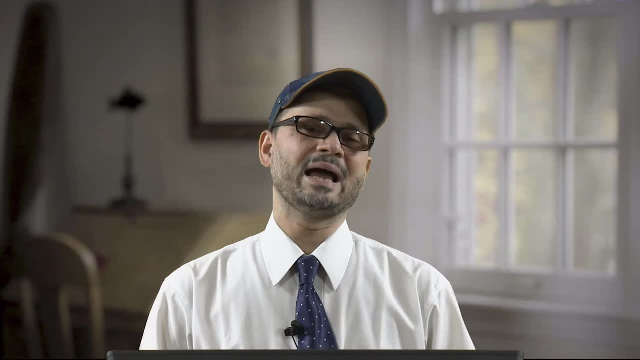 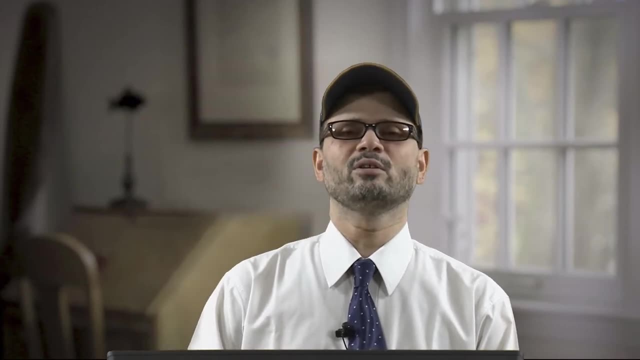 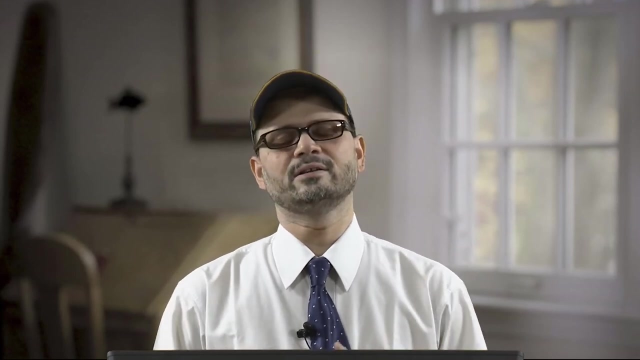 have the deposition of the metal at one of the cathode and that is very, very pure, you know, in pure form. So basically you can also control these parameters for increasing the rate of deposition and that can be done. So electrode position controlled is controlled. 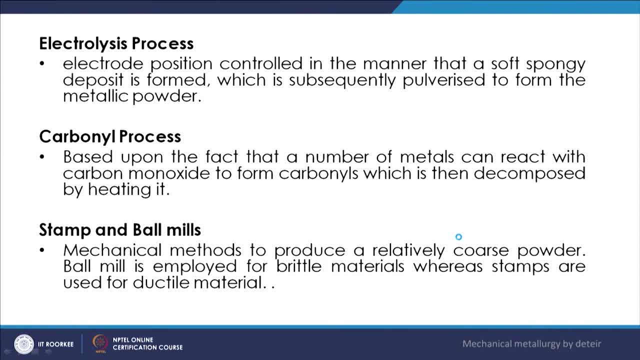 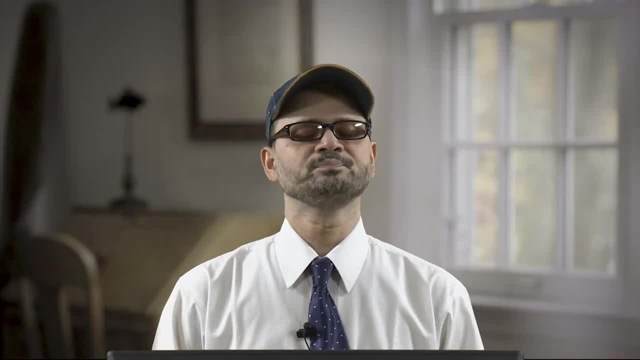 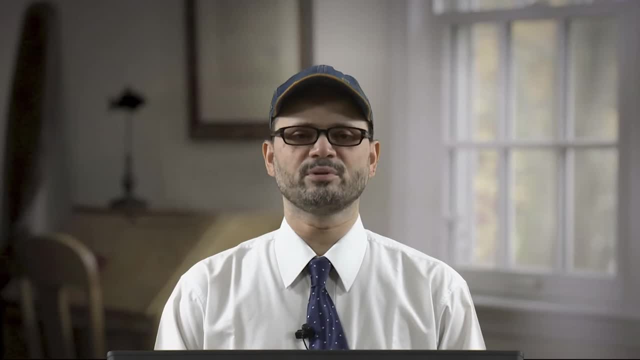 in such a manner that soft spongy deposit is formed on one of the electrode And then you can take that and then you can pulverize it, you can crush it to powders and use it. So this electrolysis process, So electrolysis process, is a very important process to get you the pure metal you know. 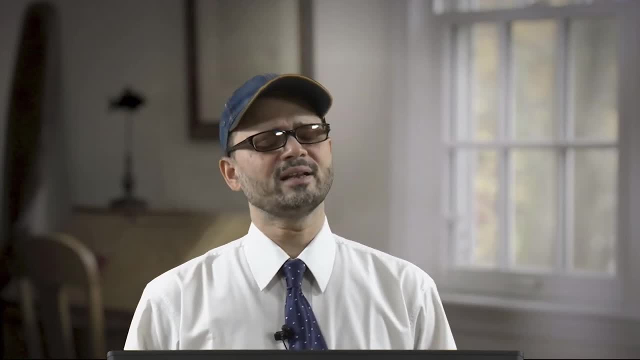 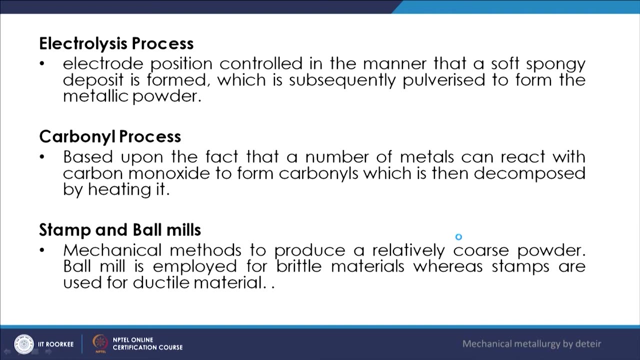 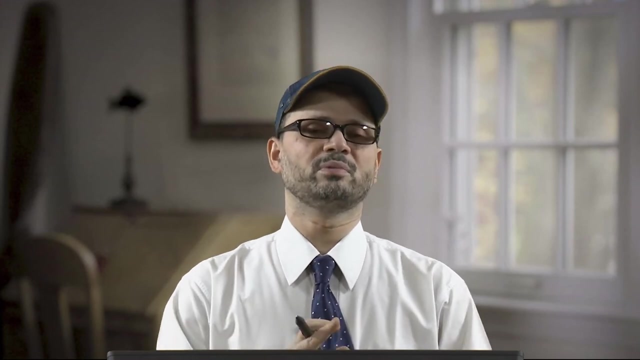 production. There is another process that is known as carbonyl process. So here, basically, the metal carbonyl is there and that will be decomposed by heating it. So once you decompose it by heating, then it will be forming to the process. 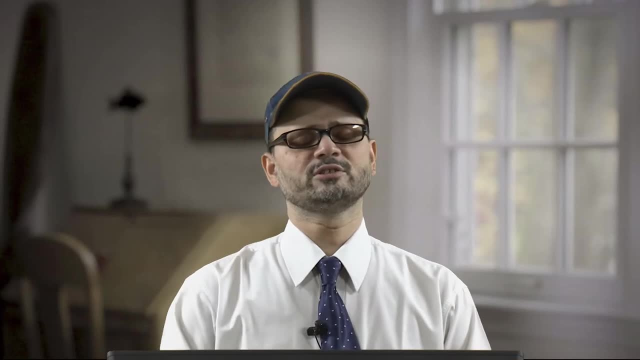 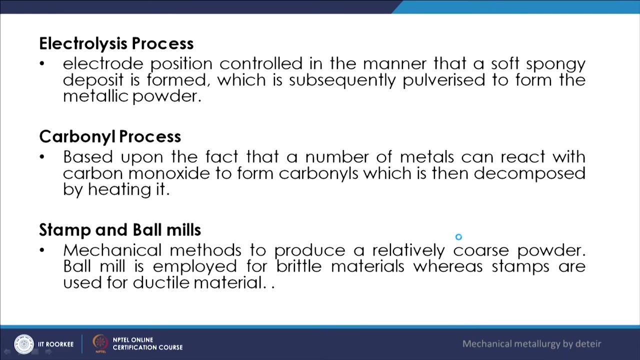 So it is based upon the fact that a number of metals- what happens? they basically react with carbon monoxide to form the carbonyl and then it is decomposed. So we will have some more study about it. Then stamp and ball mills, So this may process. 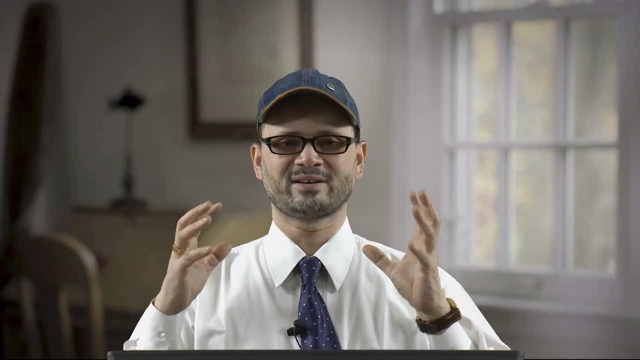 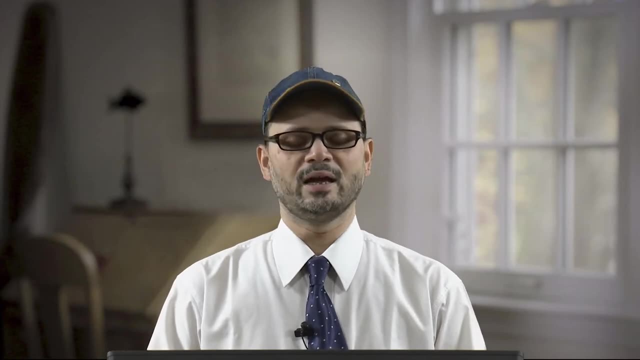 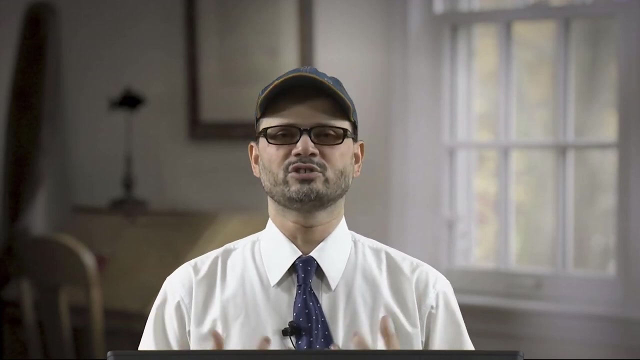 is about basically, you know, crushing the material and stamping for the ductile materials, So you get a meganamed solution, which is compound, from which you get the powder. So you have the mechanism by which you basically crush it in the ball mills using balls, steel balls. 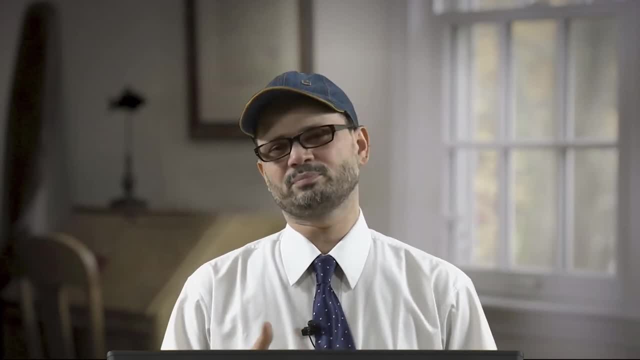 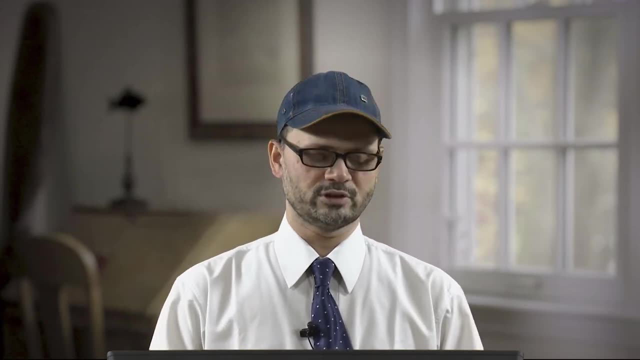 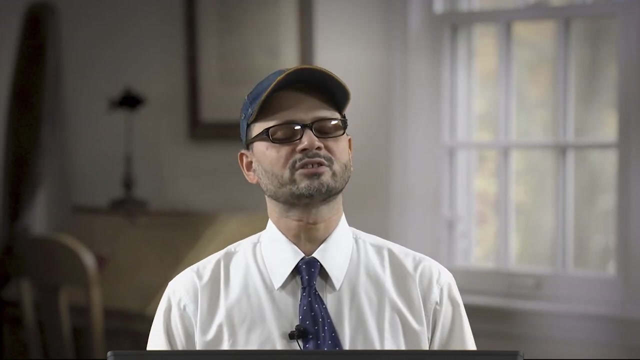 or the hard balls. So you are crushing the material, especially the. you know, crushing is used normally for the brittle materials, and when it is ductile one, you can use the stamping method. So we are discussing about the oxide reductions. Oxidized reduction 2 viel figure …헵 continue. 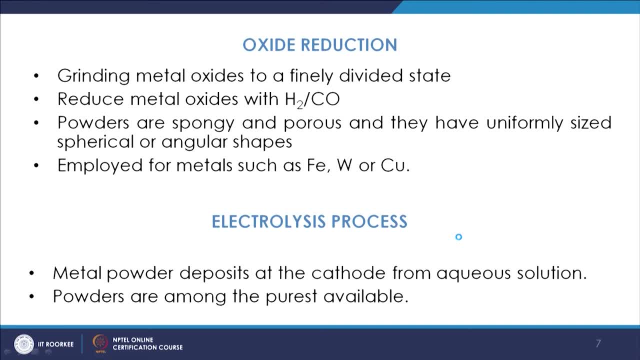 5 and having somealla is So oxide reductions. normally you have the, you can have alcohol, fructose, afford to solid站 and there are several more In the process. you actually use of hydrogen or carbon monoxide and we use that. that we have already studied. 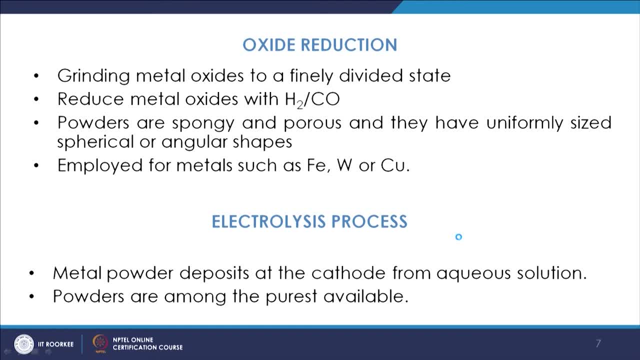 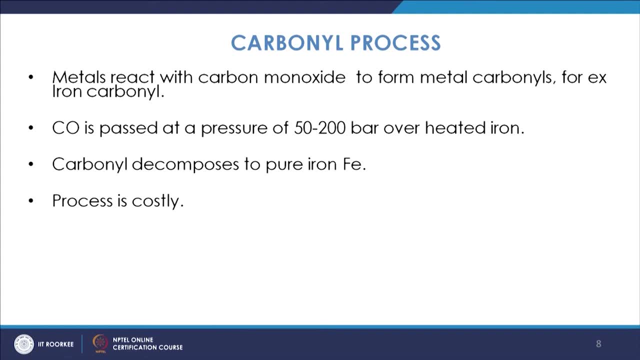 You have, you know, deposition at the cathode and they are very pure, So they are purest of the form. and in carbonyl process what happens? that CO2, carbon monoxide, is So, first of all, metal will react with carbon monoxide to form the metal, carbonyls, So the metal 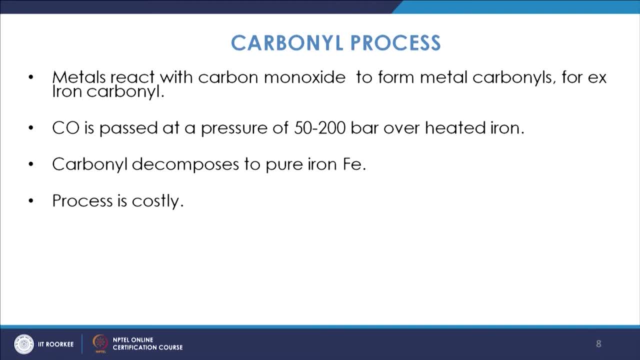 will be reacting with carbon monoxide to form the metal carbonyls, like iron carbonyl. Then the carbon monoxide will be passed at a high, very high pressure, that is, 50 to 200 bar over that heated iron, and in that process the carbonyl will decompose to pure iron. So the process. 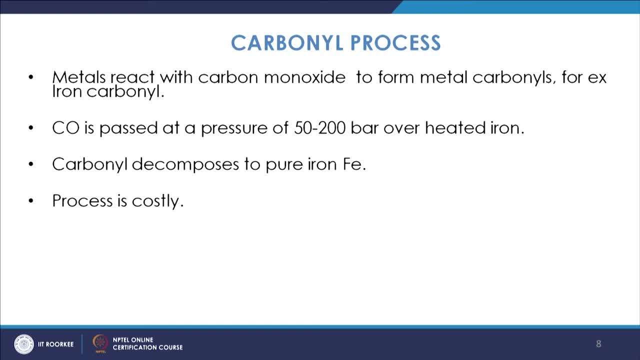 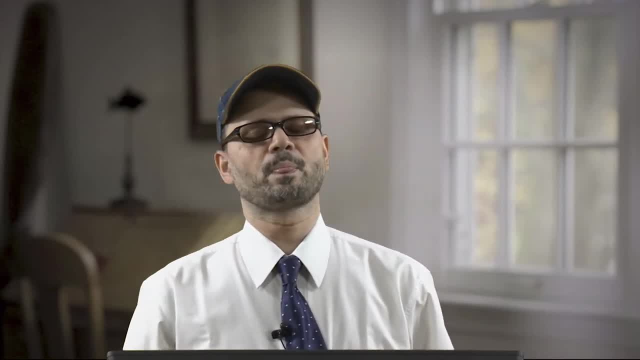 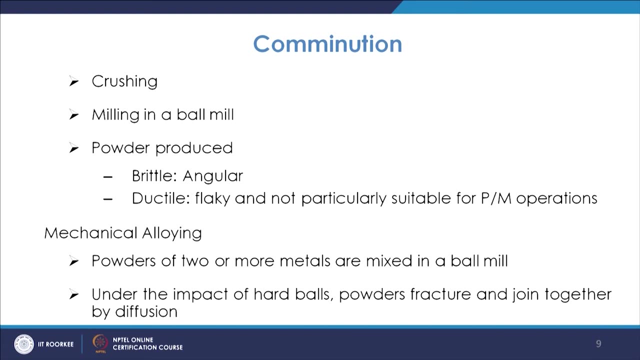 is softly, although it gives you pure, you know powder, but it is costly process. Another process which is important For making the powders is comminution methods Now, in that, basically, you have the crushing of the metal and that way you can get the powders, So you have milling in a ball mill. 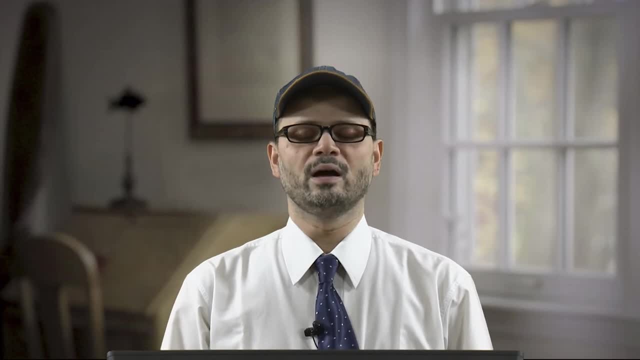 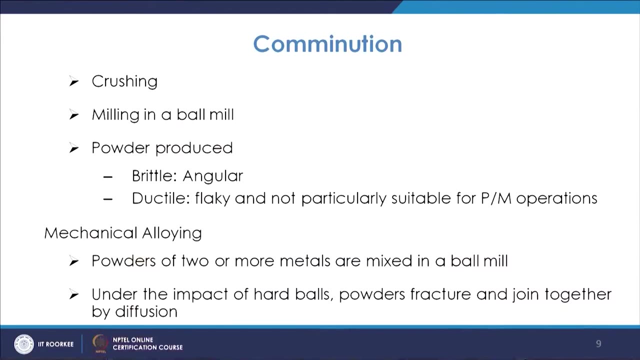 and powder will be produced. and for that what happens? that the if you have the powder which is of made of The brittle material, then you can get the angular type of powders, but if you have a ductile material you can have the flaky, which is not very much suited for the powder metallurgy. 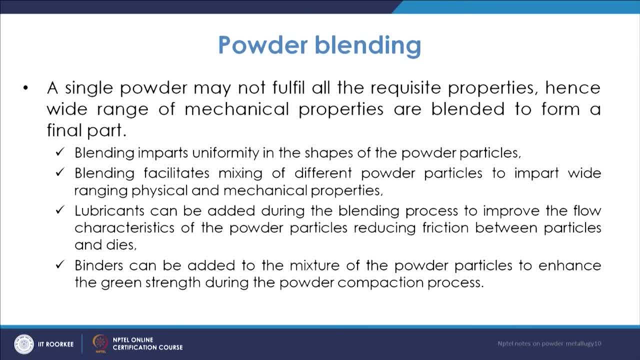 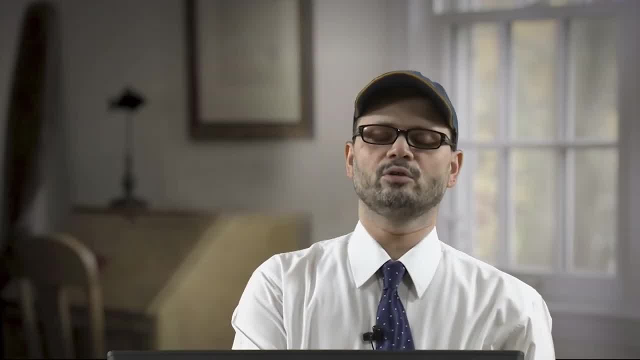 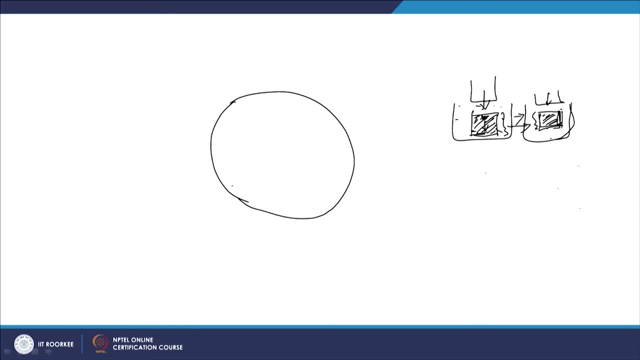 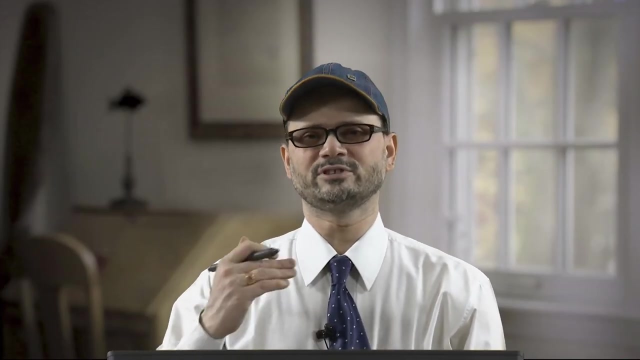 operations. So this is how you know we go. So what happens that in normally in a you have a you know ball mill So you have a very large type of You know powders. So you must have the idea about this process if you have visited certain 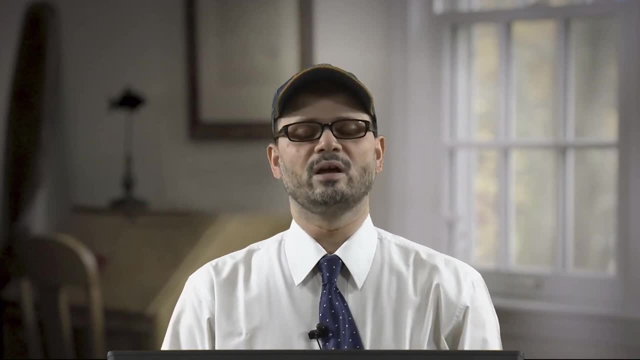 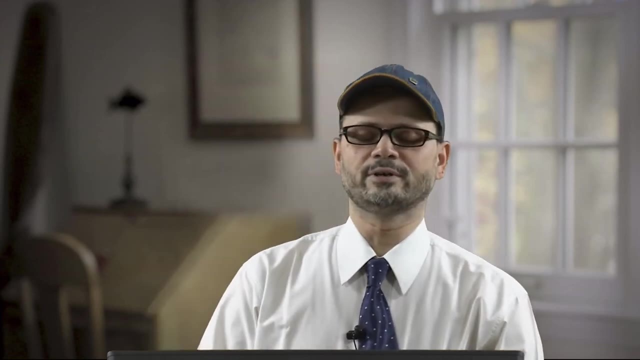 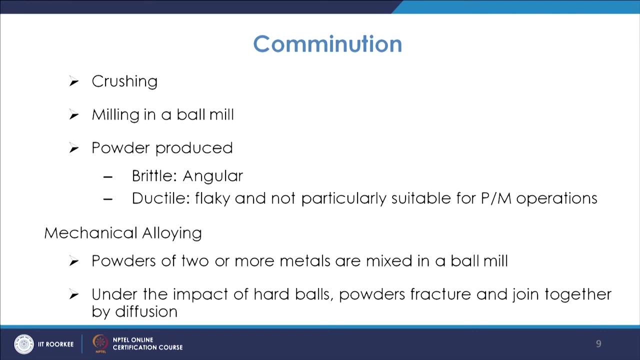 steel plants or thermal power plants. there also you have a ball mill plant where you they pulverize the coals and all that. So you have, that is the process- Mechanical alloying, so that is, powders of 2 or more metals are mixed in a ball mill. So if in the ball mill 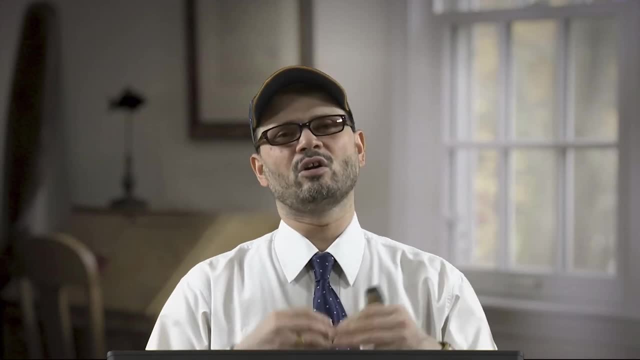 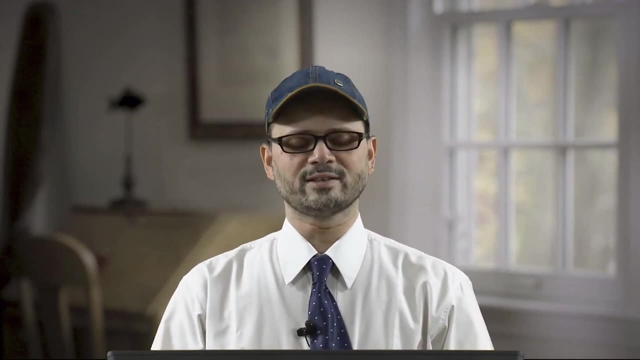 you have the powders of 2 or more metals, Or if you put 2 or more metals, then they will be crushed and then they will be alloyed also or mixed also. So under the impact of the hard balls, these powders failure, fracture. 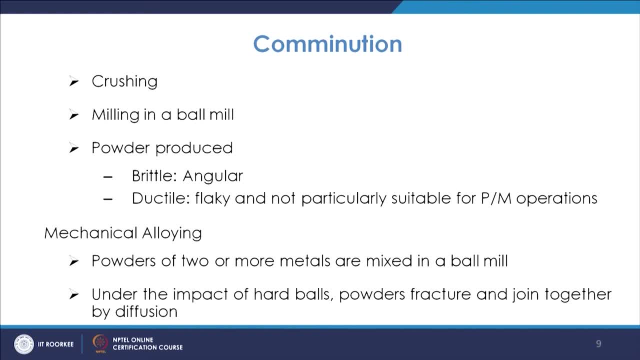 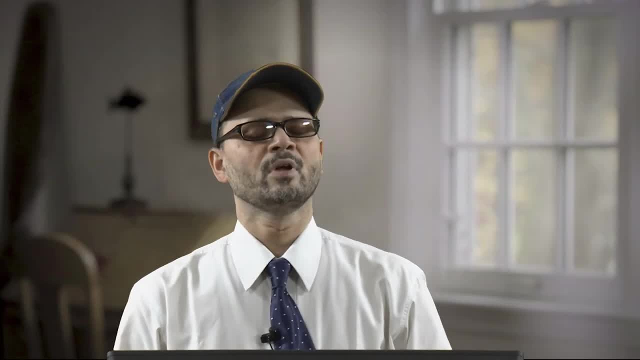 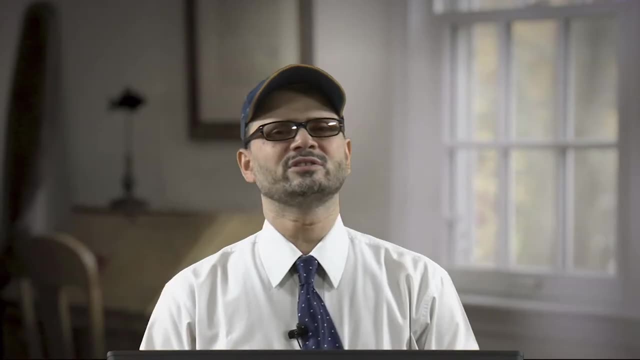 and joined together by the diffusion. So that also is possible under the action of this impacts. So they join also by diffusion, Now powder blending. So what happens that you? it is not always required that you. 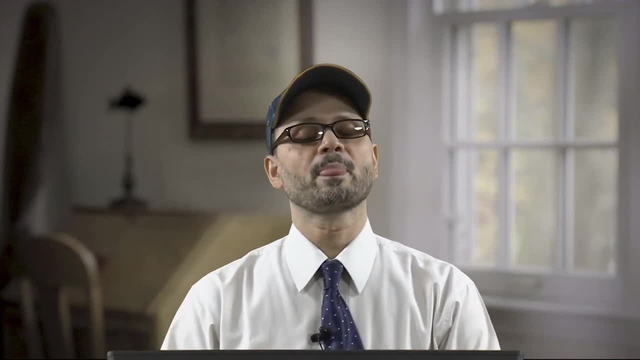 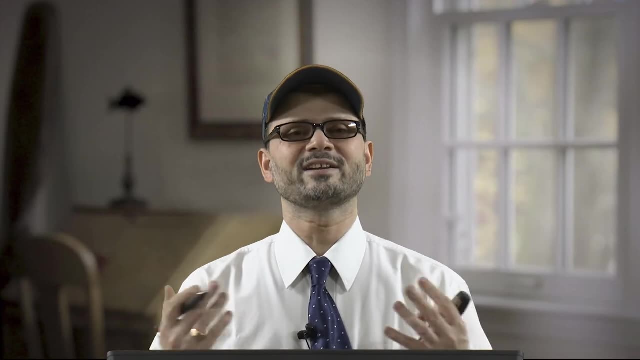 You can work only with the one kind of powder. So basically, you know a single powder may not fulfill all the requisite properties, So you require basically the wide range of mechanical properties which will be available by the use of different types of powders. 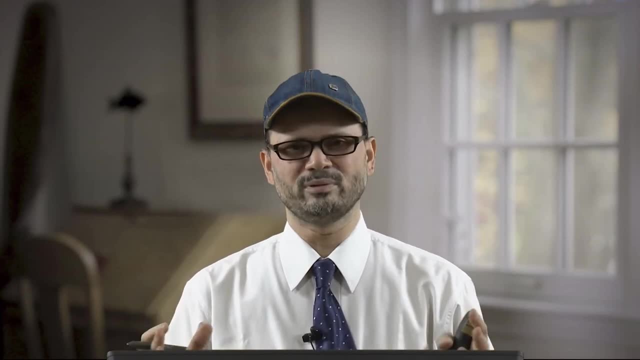 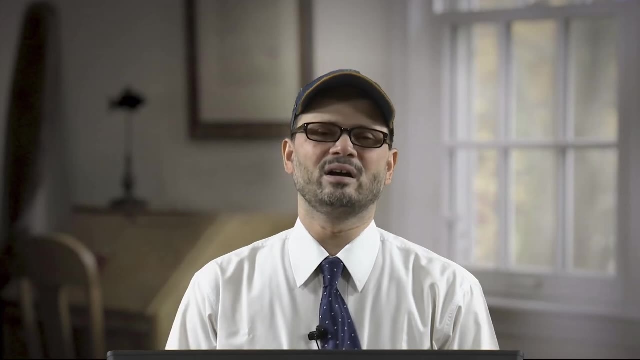 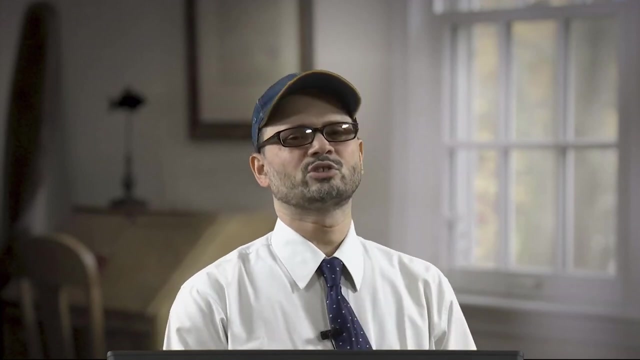 So the, basically, they need to be blended. they will need to be mixed properly, in proportion, So that you get the requisite type of properties, like some may give you, you know, Better strength, some may give you better, you know, resistance to corrosion and all. 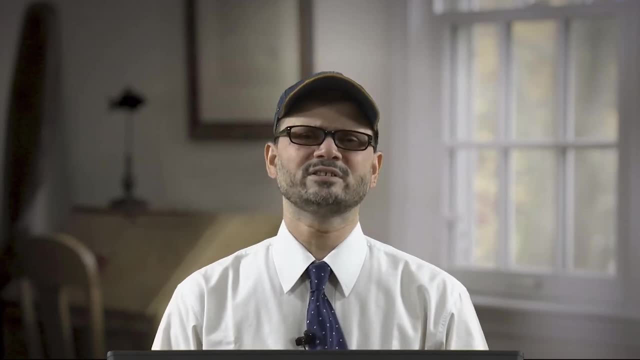 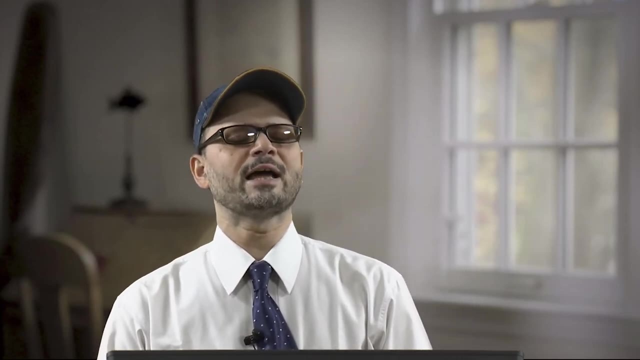 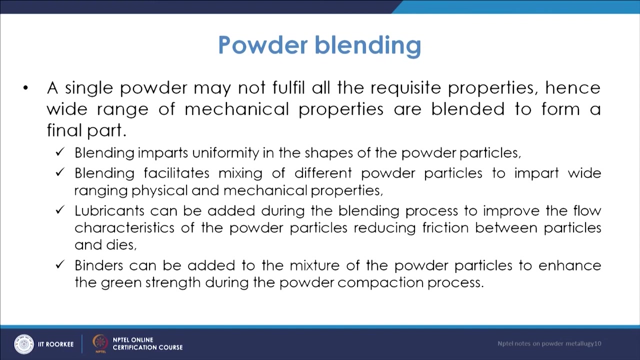 that. So the different powders may have the different properties, and that is basically attributing towards the final product preparation. So for that the blending is important and blending will be imparting uniformity in the shape of the powder particles, So it will. 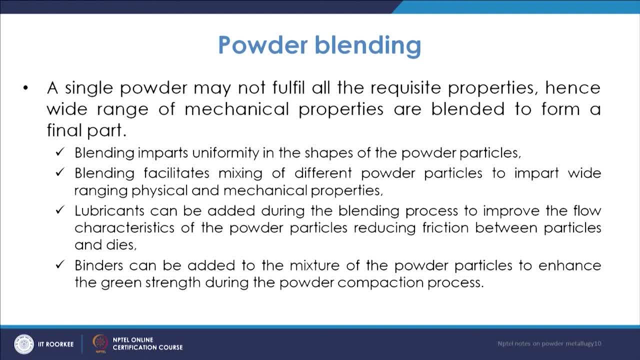 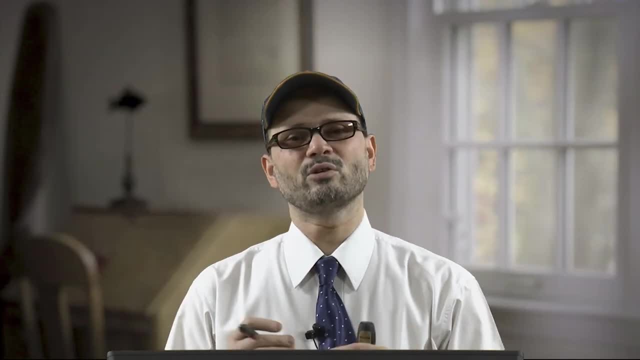 be giving you that in uniformity, Then it will be facilitating the mixing of different powder particles To impart wide ranging physical and mechanical properties. So, as we discussed that when you have the mixing of the different proper, you know powders of different properties. 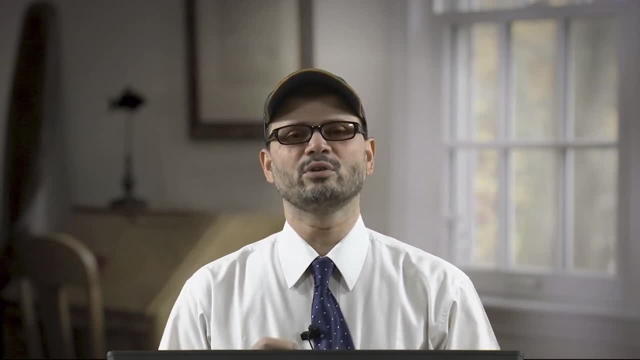 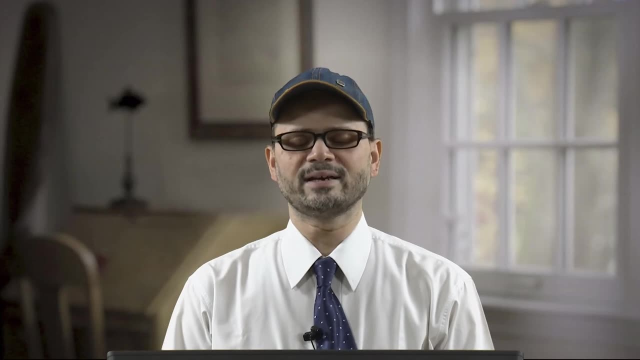 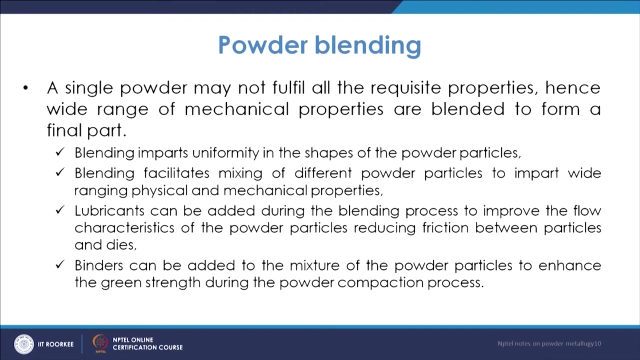 then certainly they are. you are going to achieve better physical and mechanical properties. Lubricants can be added during the blending process to improve the flow characteristics of the powder particles, So it is reducing friction between particles and dyes. Now, while blending, you require the 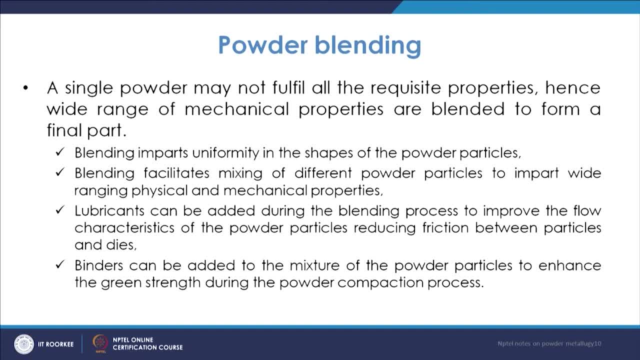 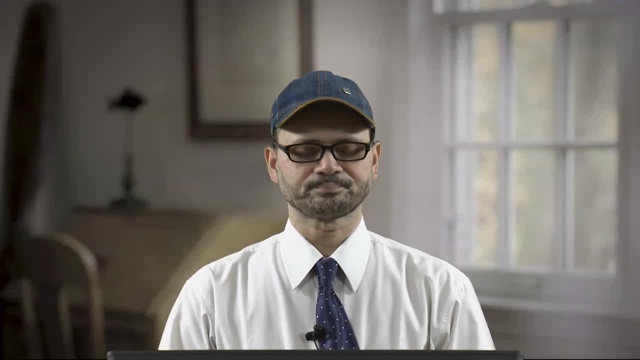 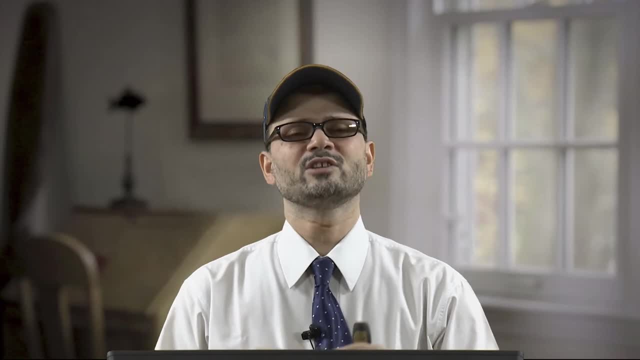 use of certain type of lubricants So that when you are, you know, blending, the flow ability should be better, and in between the particle and the dyes, when they are, you know, having that relative motion between them, there should be minimum friction So that the mixing process 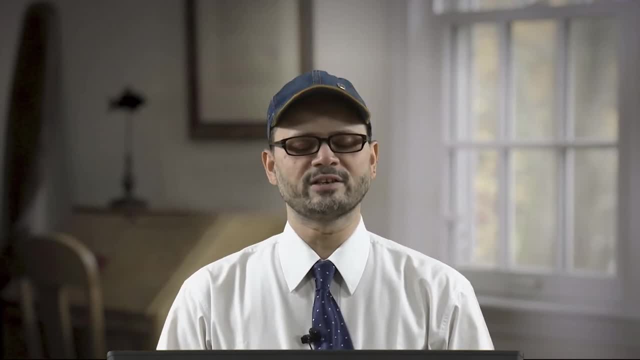 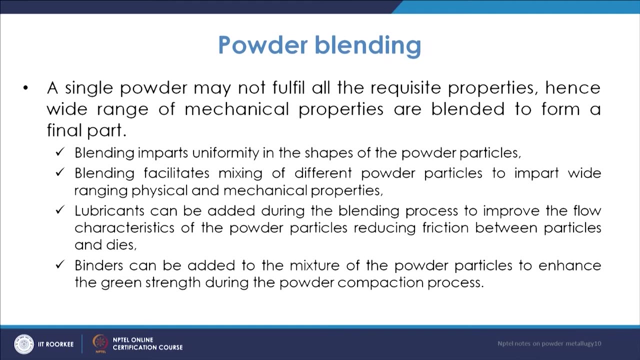 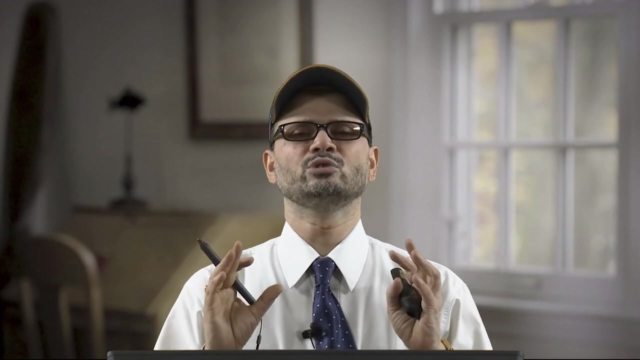 is more effective. So for that the lubricant is added and also you add the binders, which are added to the mixture of the powder particles to enhance the green strength during powder compaction process. So basically, as we discussed earlier, also you use certain binders- may be water. 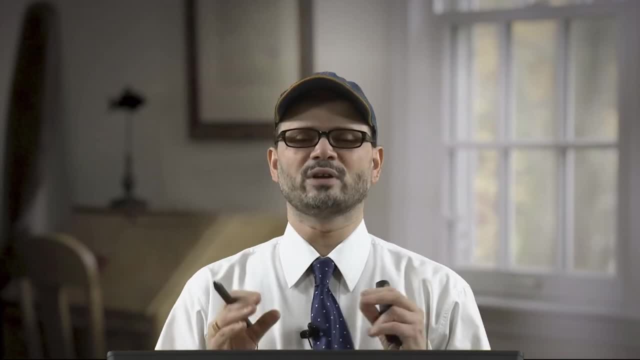 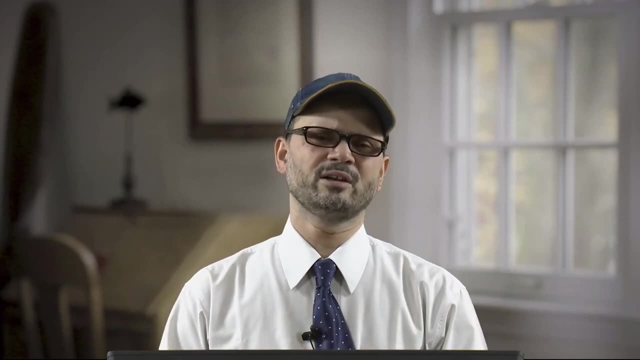 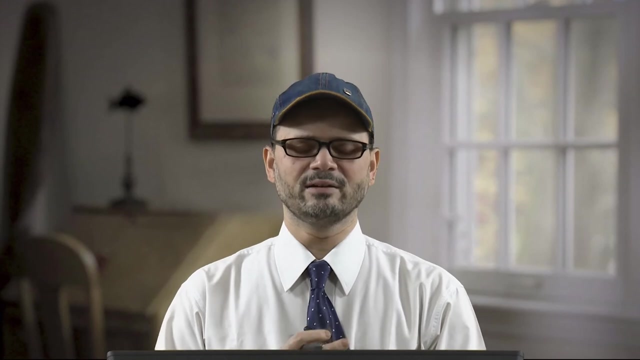 based or even not water based, So you can use the these binders to so that they are, you know they are. cohesion develops, cohesion between the particles. cohesion develops. cohesion between the powders develops, or the, you know, attraction between the different powders develops. And basically, from that way you increase the green strength of the compact and then further you are going to do the compaction so that time you will have more and more increase in the compactness of the specimen. So these binders are useful for the powder blending. 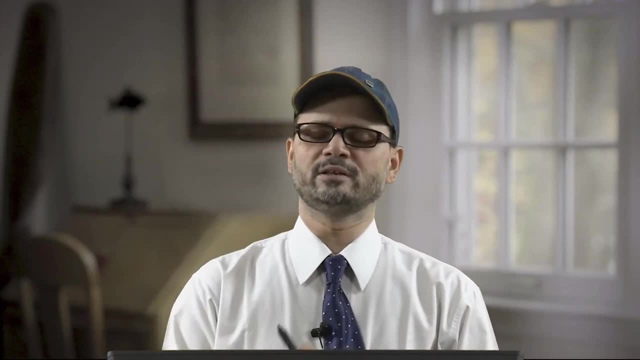 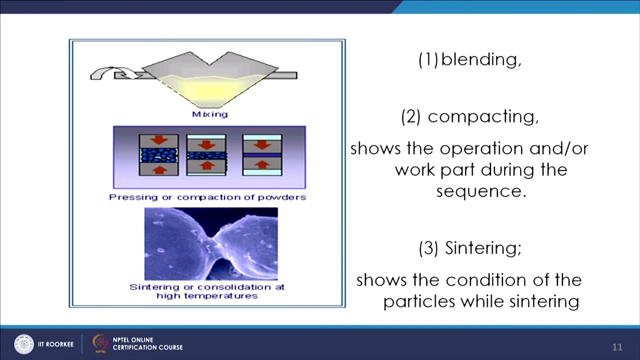 So this process talks about the blending. then once you do the blending, then you are going to compact it. so for compacting, you apply this pressure and you so highly compacting. you can see that the space between them is there, that is decreasing and that is further. 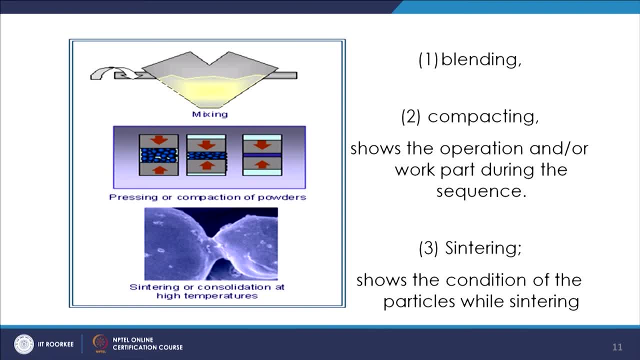 decreasing. So that way you can change the spacing between the particles as the compaction is done, And then ultimately you go for the sintering. so when it will be sintering, then during the sintering or the consolidation, when the high temperature goes, there will be bounding developed. 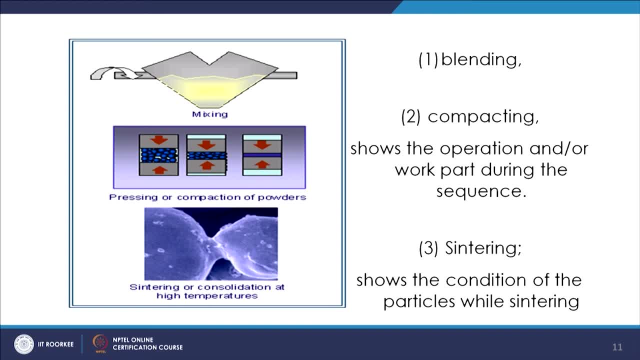 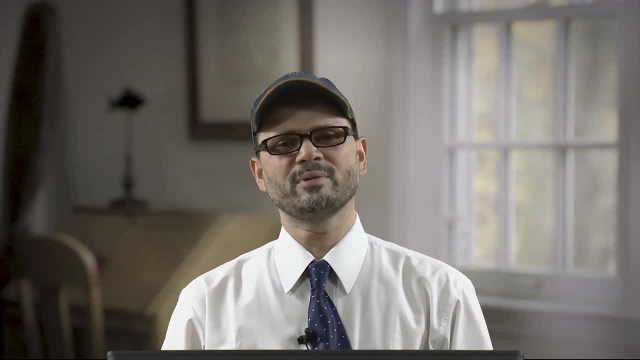 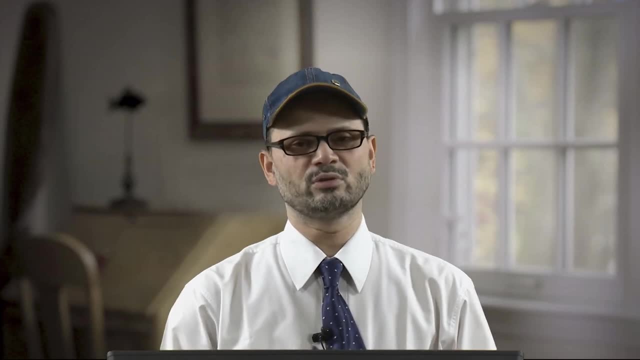 initially. So bounding will be developed and that way the material in between the material, whatever porosity is there, that is gone. volatile materials will be coming out and porosity anyway is maintained, whatever you have to maintain that way, But volatile materials will go out and then there will be consolidation, there will be 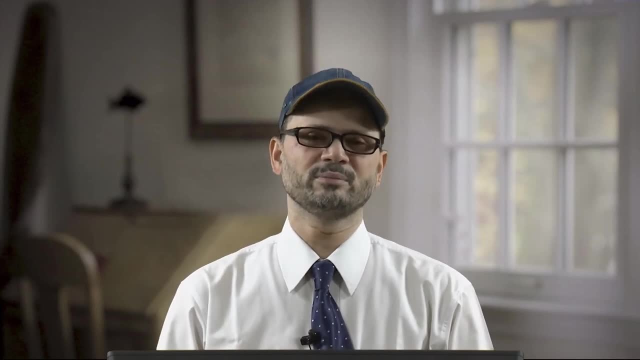 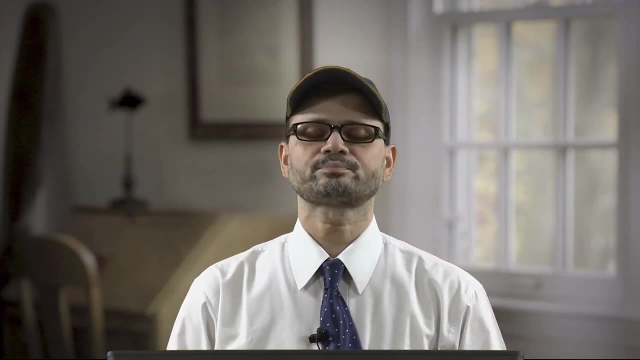 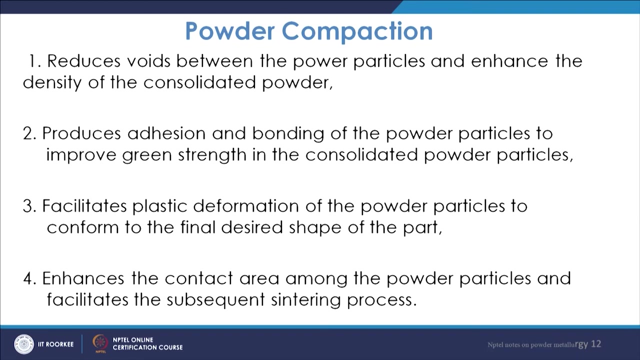 increase in the strength. there will be bounding, you know, fusion of the materials, powders, with each other, So that way your strength is developed. Now, what is a powder compaction, basically, so powder compaction is required because it will be reducing the void between the powder particles and enhance the density of the consolidated 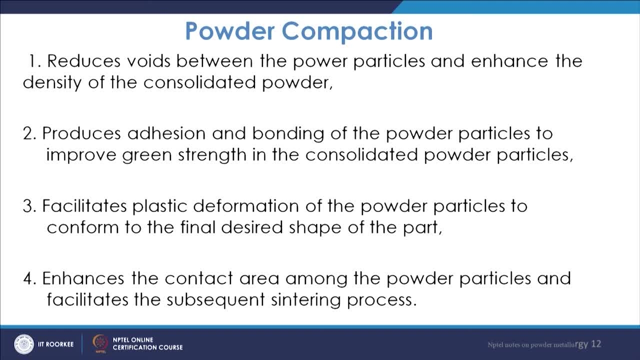 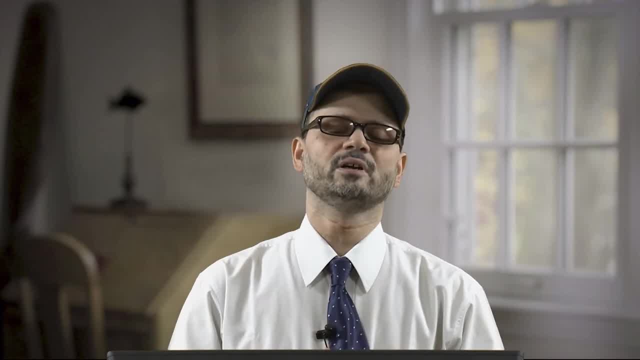 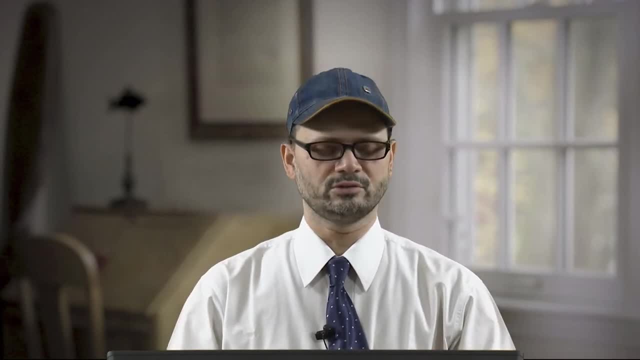 powder. So once you have the powder, then you have you and you have blended it and you have made the compact. now you have to increase the density of the- you know- consolidated powder, because otherwise you have a large- you know- inter particle spaces between them and that needs. to be basically reduced and it will be ideally coming to that when it is, there is ideal inter term distance. So, as per their crystal structure, so as you increase the compaction pressure, or as you increase the degree of compaction, then they are. the spaces between them is basically. reduced and the void between the powder particles will be, you know, reduced and the density will be increased. produces adhesion and bounding of the powder, of the powder particles, to improve green strength in the consolidated powder particles. So again, that is to for improving the green strength, facilitates plastic deformation of. 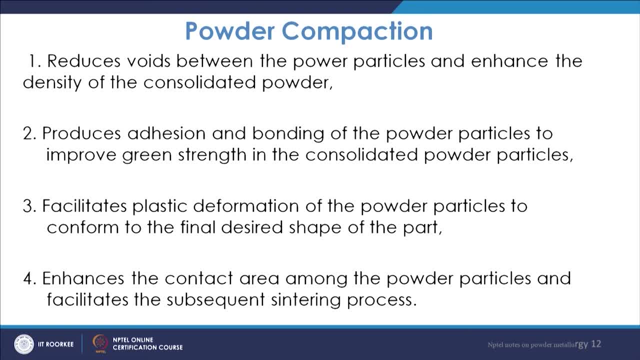 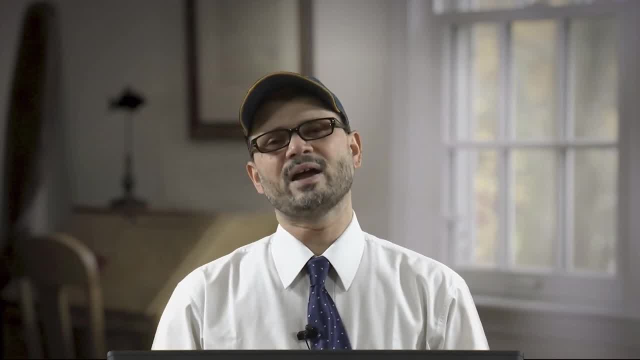 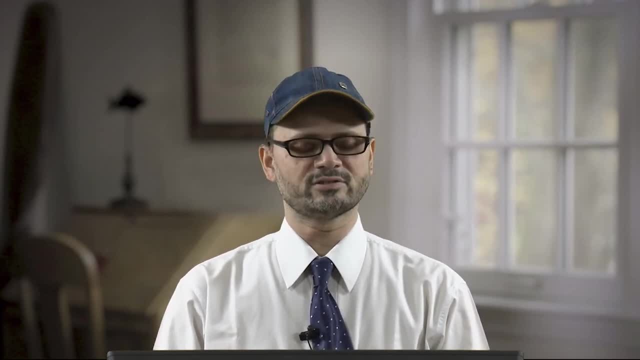 the powder particles to conform to the final desired shape of the product. So what happens? that when you do the compaction then there will be plastic deformation of the material and it will be coming to the final desired shape of the part. Enhances the contact area among the powder particles and facilitates the subsequent sintering. 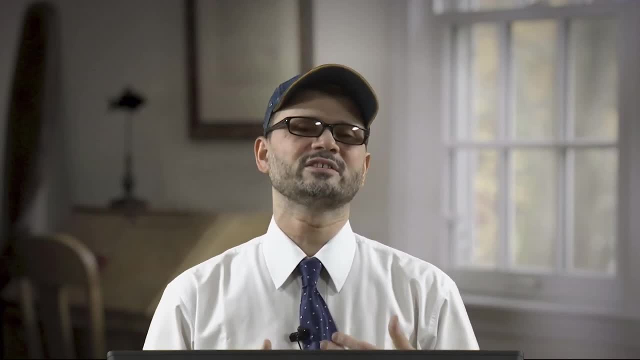 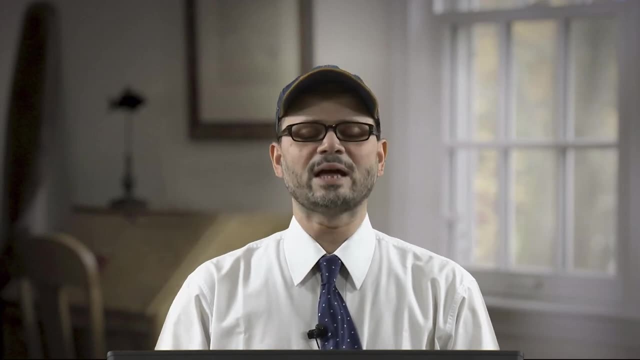 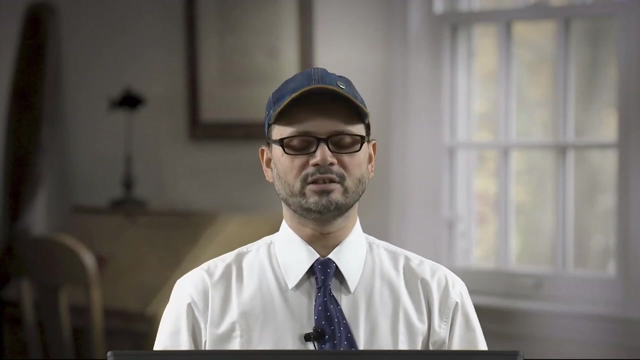 process. So the contact area between them will be increasing, increasing and that will basically be facilitating the subsequent sintering process. So that is the you know about the powder compaction. So if you can see this compaction sequence how it is done, you see that you have the start. 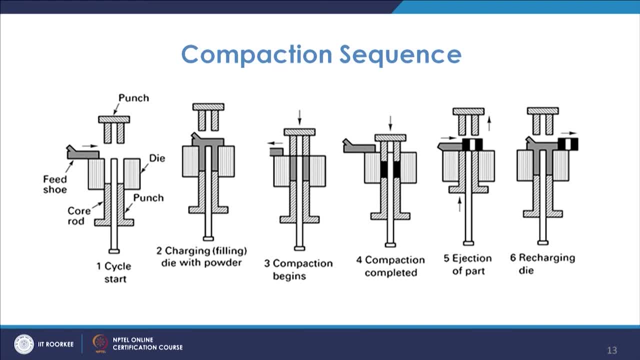 of the cycle where you have this is the dye and in that, basically, you have this is the cavity in which this material is kept and the powder is kept, And then, from the top, you will have the punch, the top part will come and it will apply the 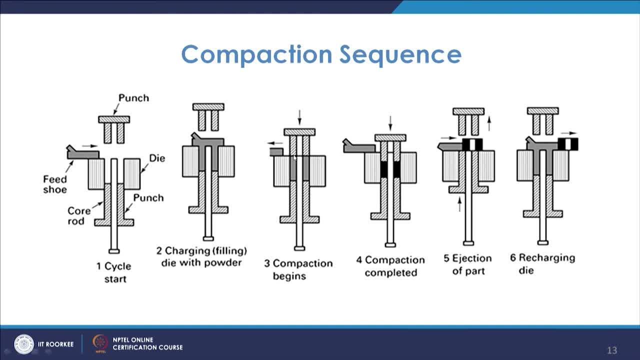 pressure, So a dimension or a height of this much So. here you have the start of the cycle, then you have filling the dye with the powder, Then the compaction has started, and once you have compaction started, then the height of this specimen will go on decreasing. 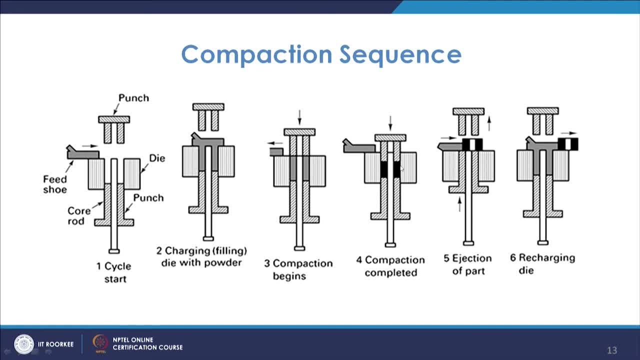 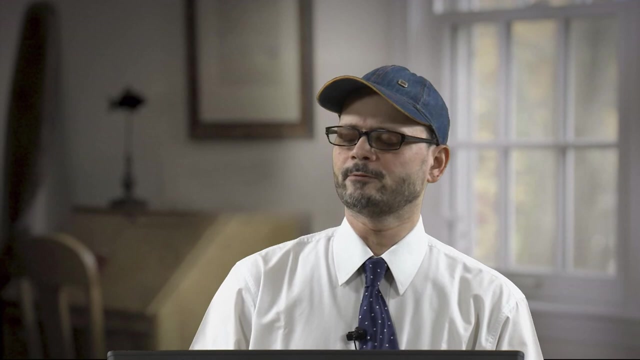 And it will be decreasing to this level and then, once you have gone, you have reduced the height to certain level, Then basically you have to take this punch out and then you are getting this final product with the height which is required for you. So that is how these you know, compaction is done in sequence. 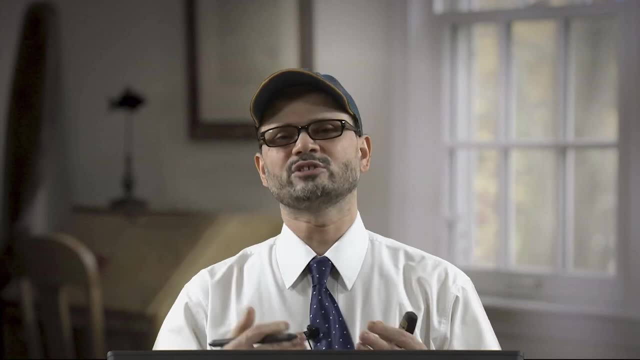 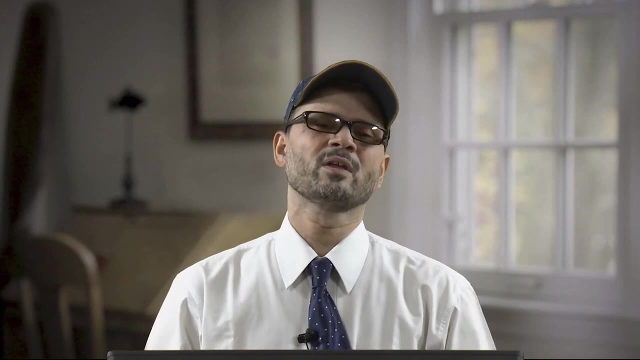 And then further you have the final product And further, after one sequence, you are going to further repeat the process. So that is how the compaction is done, and you can see that the dimension is reduced and the density will certainly be increasing in that time. 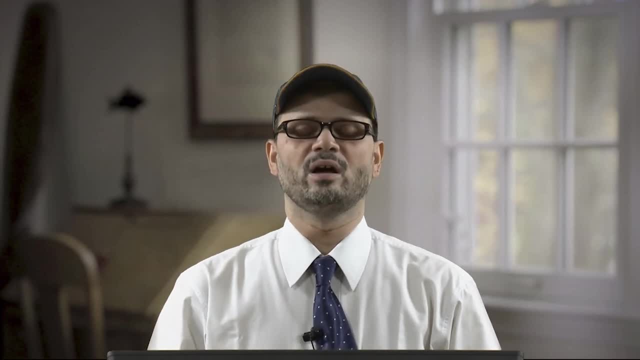 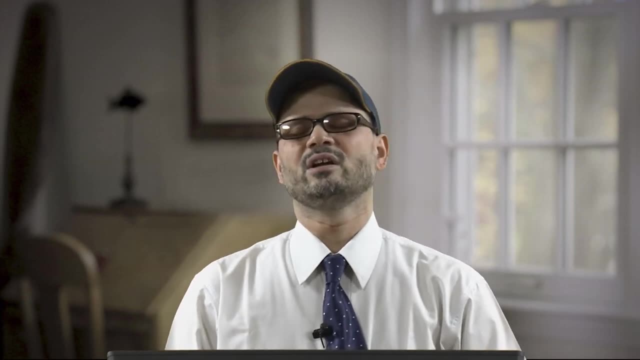 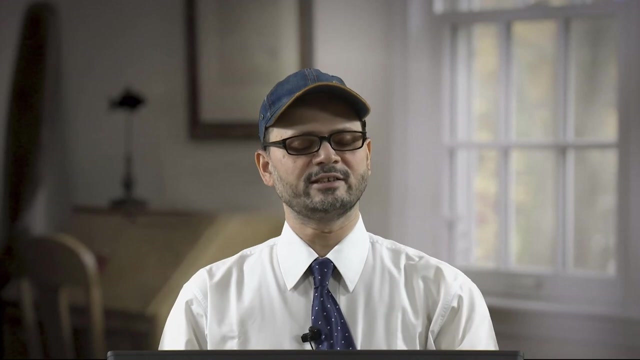 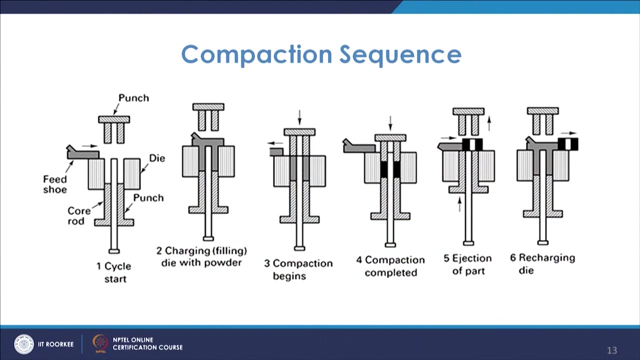 So that is the sequence of compaction which is, you know, done in the case of the powder metallurgy. Now we also do the compaction. may be sometimes we are doing the compaction here, But what we see here, in this case, this portion may be, you know, this part may be, you know, stationary.